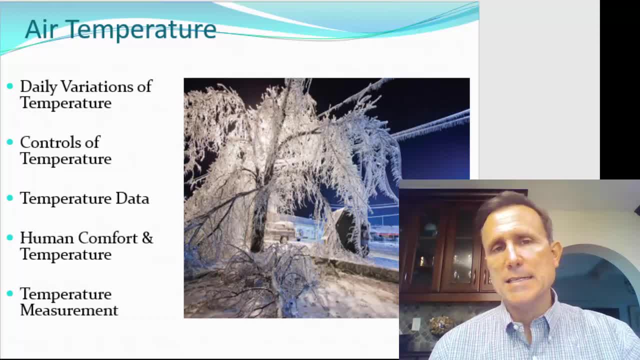 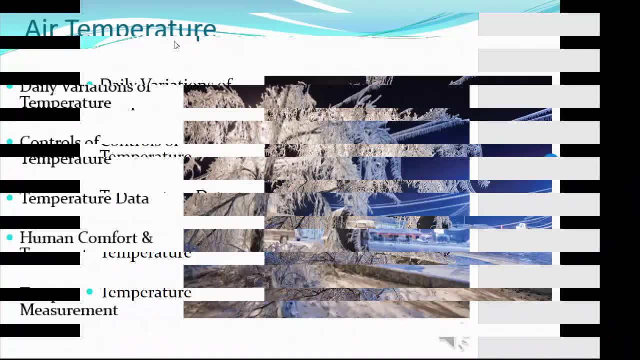 look at human comfort and temperature, wind chills and heat indexes, and we'll also briefly talk about temperature measurement. But first we'll take a look at the daily variations of temperature. The daily variations of temperature. We know that the atmosphere is heated from. 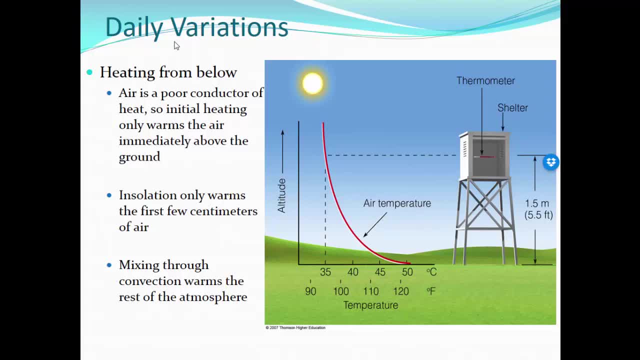 below The atmosphere acts as a window or is essentially transparent to the sun's incoming shortwave radiation. that insulation from the sun, The shortwave radiation of the sun, moves through the atmosphere, some of it being absorbed- very little, some of it being 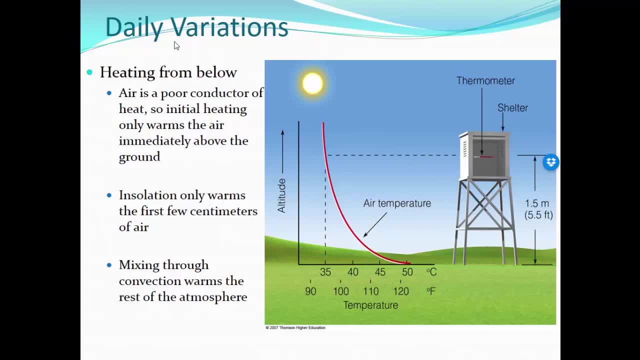 scattered, Some of it being reflected, but most of it reaches the ground. The earth absorbs that radiation. The earth is warmed and then radiates away longwave radiation that is absorbed by selective absorbers or greenhouse gases, But the main warming of the atmosphere occurs. 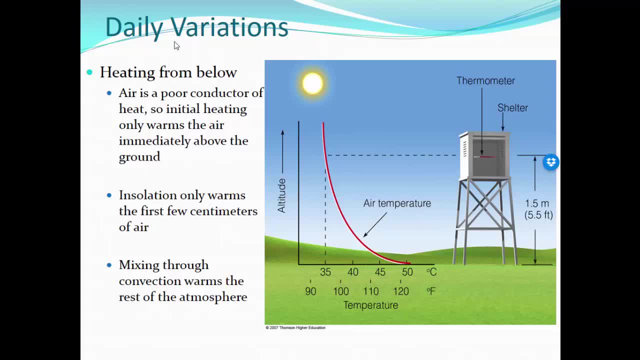 from below as the warm earth heats the first few centimeters of air, and those first few centimeters of air then rise or lift by convection To warm the rest of the atmosphere. And because that occurs, the atmosphere is heated from below. And as you look at our illustration, one thing to point out here is that box up. 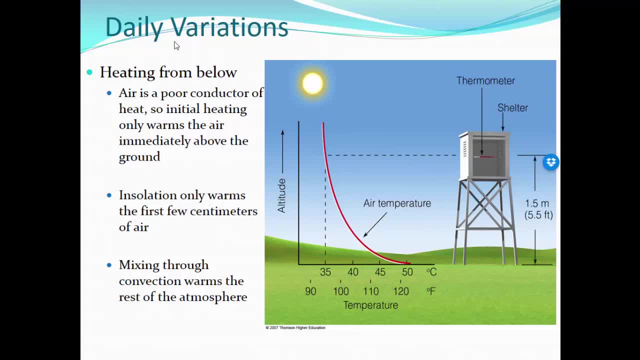 on legs, that wooden box with a thermometer in the middle of it. that is actually the correct way to measure the temperature. It has to be six feet off the ground. it has to be inside a wooden box, the thermometer, away from all the walls. there has to be wooden. 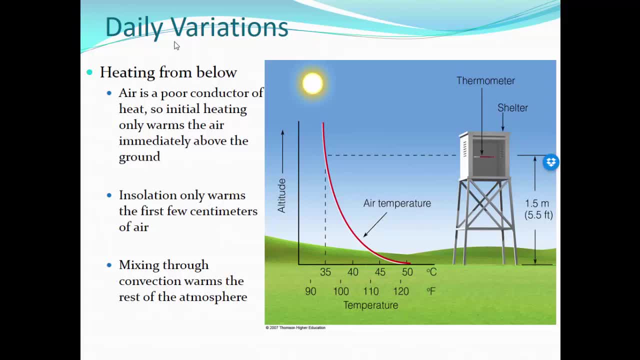 slots to let the air go through, And that is how temperatures are measured. It has to. Temperature is is measured all across the country and really all across the globe. now in the last 10 to 15 years, Digital temperature measurements have began to change that, but that's how it was done. 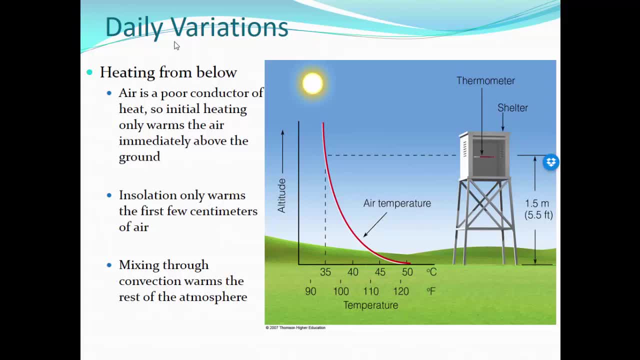 literally for centuries, and looking at the graph, with the Y axis being altitude and the x-axis being temperature, we see at the surface the temperature somewhere just above 50 degrees Celsius, and in the first few meters of the atmosphere that temperature drops just over 15 degrees Celsius, because you're always going to be warmer during the daytime. 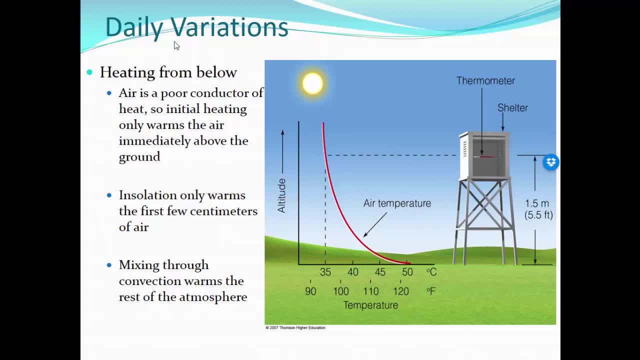 Closest to the Earth's surface. and why is that? air is a poor conductor of heat. It does not have good Thermal capacity, doesn't have good properties moving heat, thermal conductivity. So initial heating only warms the air immediately above the ground. So the initial heating of the ground, 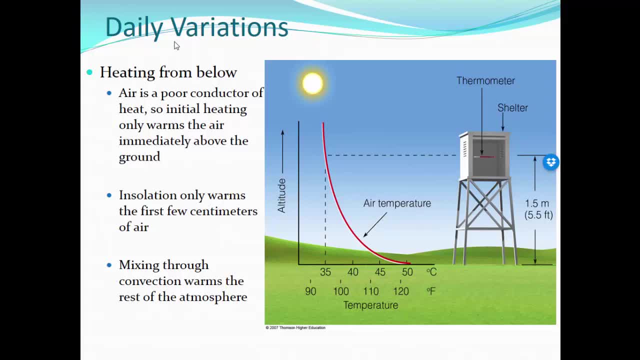 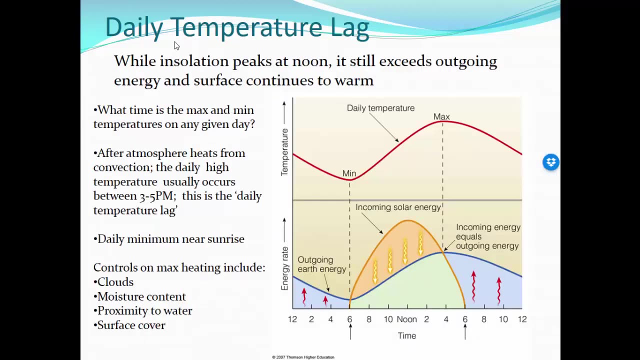 Warms the air and those first couple of centimeters insulation Warms those first few centimeters of the air and then that air is mixed through convection again, The up and down motion of the air, and that warms the rest of the atmosphere. So there is this daily temperature lag. 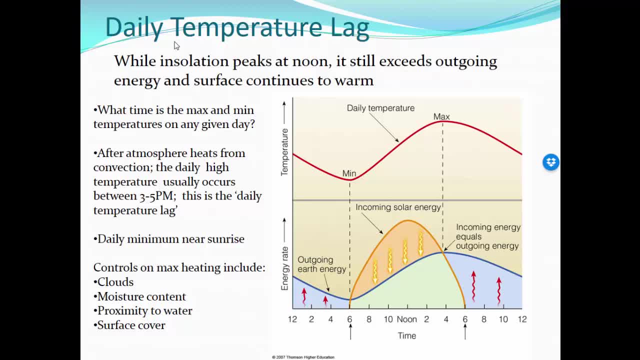 while Insulation, incoming shortwave radiation or incoming solar radiation peaks at noon. noon is going to be when the Sun is highest in the sky. It still exceeds outgoing energy Throughout the afternoon and the surface continues to warm. So look at our graph and once again, the y-axis has both energy rate and temperature, and the x-axis 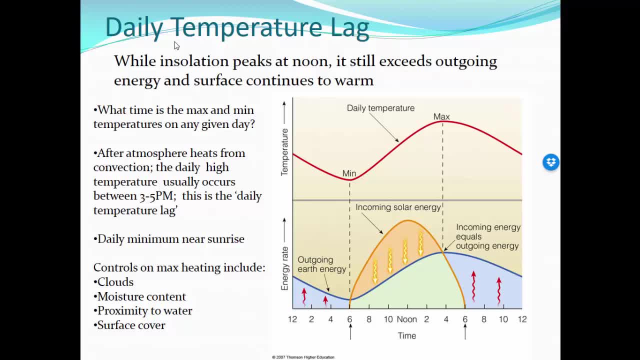 Showing the time from midnight through noon and then back to midnight and the incoming solar radiation. We're going to assume the Sun rises at 6 in the morning and sets at 6 in the evening, with the peak incoming solar radiation occurring right at noon, the highest point of the Sun in the sky- and what we see is 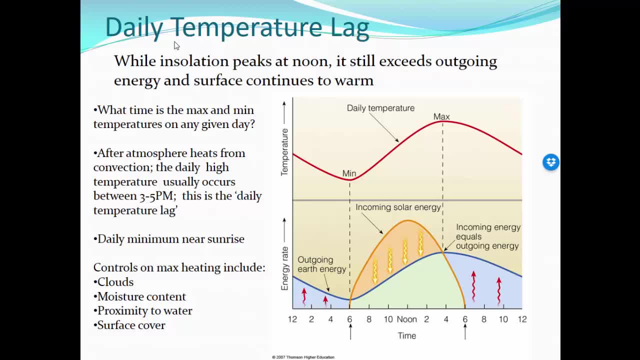 that the Earth's outgoing radiation Rises as the incoming radiation goes up as well. but the incoming radiation Remains higher than the Earth's outgoing radiation until about 3 or 4 o'clock in the afternoon, So cooling only occurs Evening or nighttime. cooling only occurs when the Earth's outgoing longwave radiation exceeds the sun's incoming shortwave radiation. 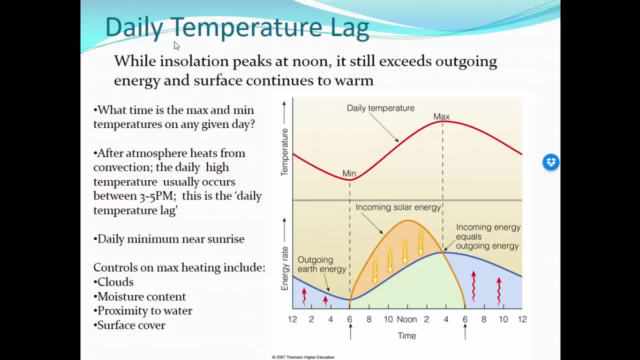 So what time is the maximum and minimum temperature On any given day? After the atmosphere heats from convection, the daily high temperature usually occurs between about 3 and 5 pm, And this is known as the daily temperature lag, the lag between Maximum solar energy and the actual maximum temperature of the day. 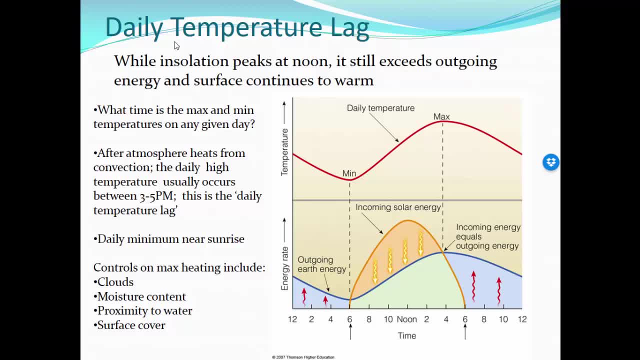 The daily minimum temperature usually happens near sunrise. now, This is not every day in all situations, but these are the generalities of temperatures: maximum and maximum and minimum. each day, as The Sun continues to heat the atmosphere and before outgoing Longwave radiation exceeds incoming shortwave radiation, the temperature continues to climb through three, four or five o'clock in the afternoon. 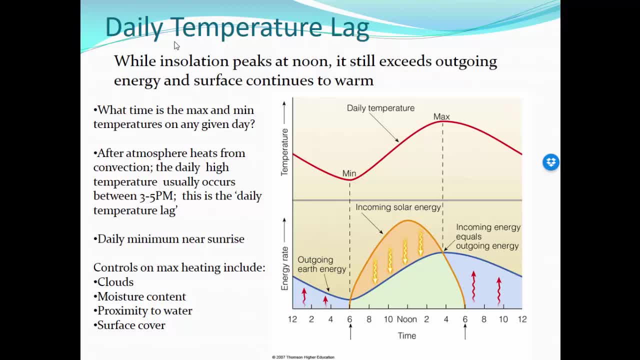 And then the temperature does not begin to fall until that outgoing radiation exceeds incoming radiation. That may happen late in the afternoon, through six or seven o'clock in the evening, But that outgoing terrestrial radiation, that outgoing longwave radiation, continues all night long, right up to Until the Sun comes up over the horizon. so cooling continues all night long, and that's why the 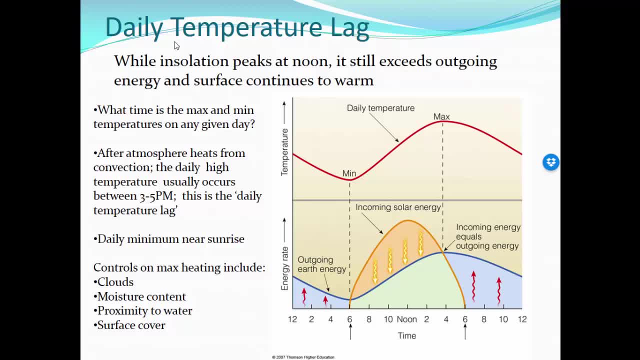 Minimum temperature typically is near sunrise. now different aspects of a cloudy day or windy day or rainy day or a cold front passage Or a warm front passage can change that, But generally high temperature the day between three and five. the low temperature near sunrise, the controls on the highest temperature of the day. 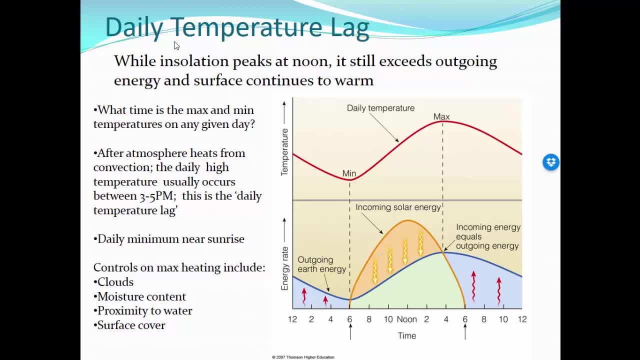 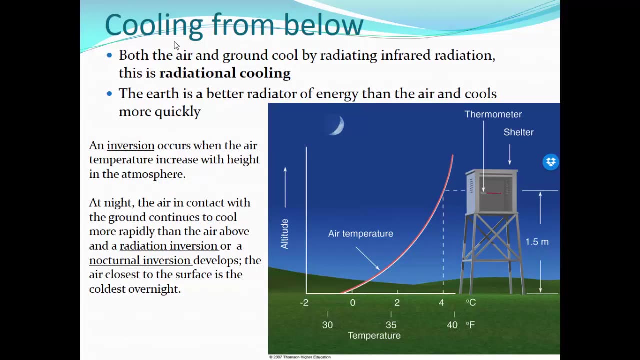 absolutely include clouds, moisture, content to the air, proximity to water and What covers the surface, whether it's asphalt and buildings, or it's waving wheat or grasses or prairies. all those things impact the daily temperature. So, in the same way that the warmest temperature was closest to the ground during the day the coolest, 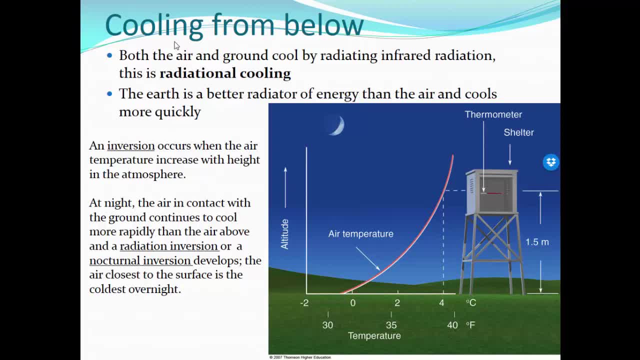 Temperature will be closest to the ground at night. Both the air and the ground cool by radiating infrared radiation, meaning the atmosphere to what degree it absorbs outgoing infrared radiation, and the earth and all the the Incoming solar radiation that's absorbed and heats up the earth. the outgoing longwave radiation of the earth and the outgoing longwave radiation of the atmosphere. 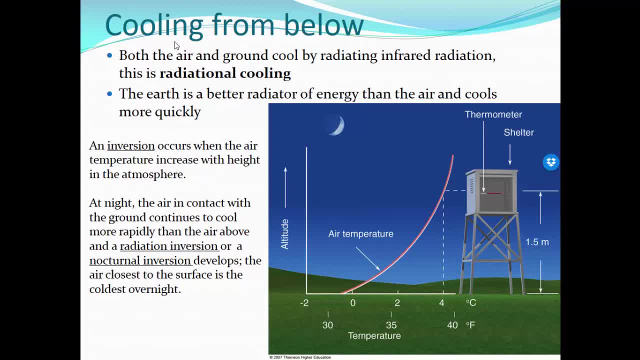 Are both moved away from the earth in the atmosphere through radiation, and that is called Radiational cooling. the earth warms up during the day and at night it just literally gives up that heat to space. now We talked about temperature decreasing with height, but in an inversion and 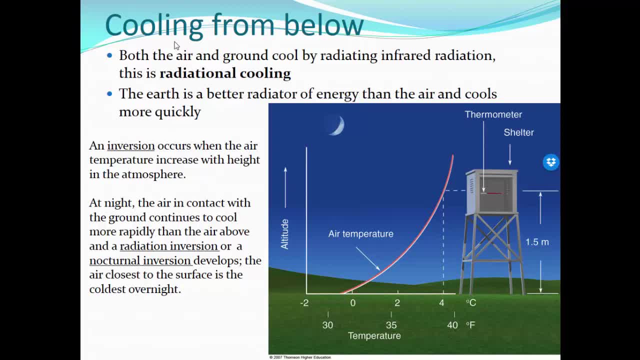 Inversion occurs when the air temperature increases with height in the atmosphere, and one of those unique and fairly small Layers where that occurs is right at the surface at night time. at night, the air in contact with the ground continues to cool more rapidly than the air above it, and a radiation inversion, or a nocturnal inversion, develops the air closest to the 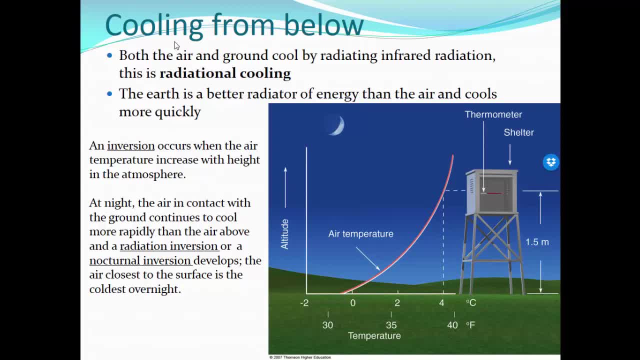 Surface is coldest overnight Because the earth is a better radiator of energy than the air and it cools more rapidly. So, while both the atmosphere and the earth cool by radiational cooling, the earth is a better Radiator of energy and it cools more quickly. so on any given very early morning, 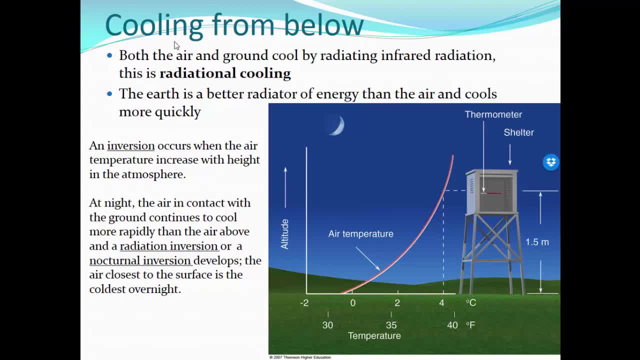 Just like this graph shows us, the temperature at the surface can literally be below freezing, while the temperature at six feet above ground level may be as warm as several degrees above freezing. and that's how you get forecasts that say overnight low of 38 degrees, but it could be some frost, because 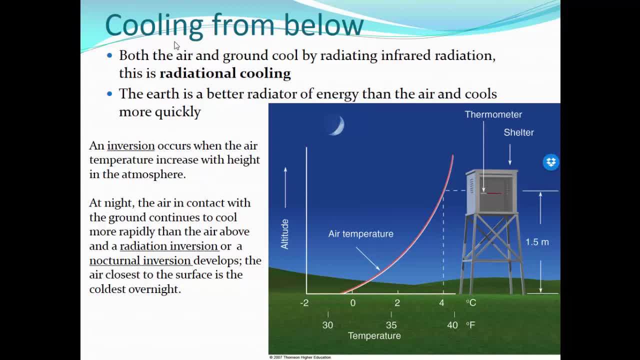 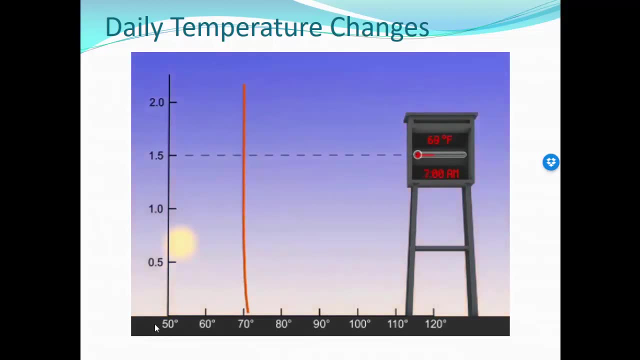 That overnight low is being measured at six feet above ground level, and the temperature at the surface could still be below freezing and allow frost formation. As the Sun rises in the morning, the Earth's surface warms more quickly than does the air above on a clear, calm day. 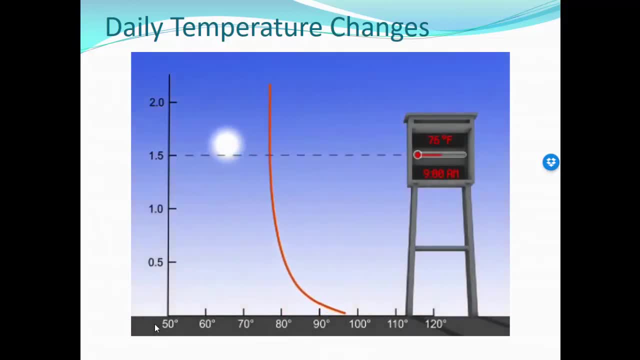 The air in contact with the surface normally reaches its highest temperature at noon, when the sun's energy is most intense. however, the air several meters Above the ground, where thermometers are usually located, typically reaches its highest temperature later in the afternoon. At night, the ground cools more quickly than the air. 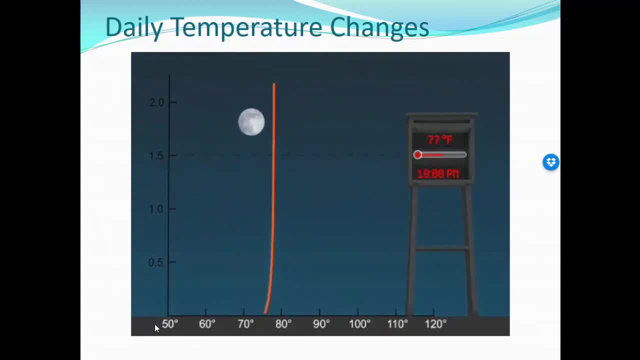 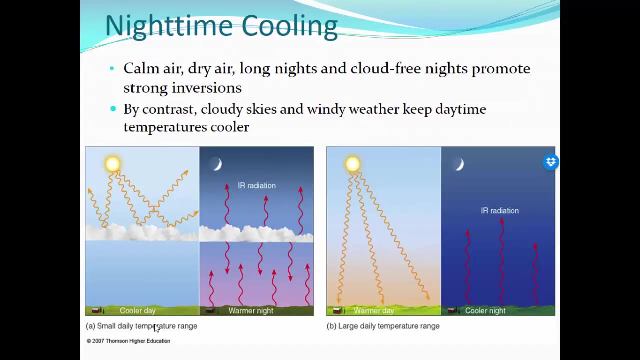 this situation causes the air in contact with the ground to become colder than the air several meters above, and The temperature inversion forms just above the Earth's surface. So, looking at both the these photos or pictures at the bottom: Calm air, dry air, long nights and cloud-free nights. 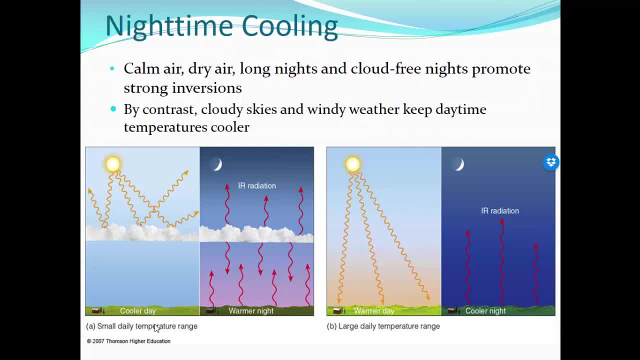 promote strong inversions or promote significant cooling. By contrast, cloudy skies and windy weather keep daytime temperatures cooler. So what allows for both day and night to be cooler than normal? Well, in the case of nighttime it's calm air, dry air, long nights and cloud-free. 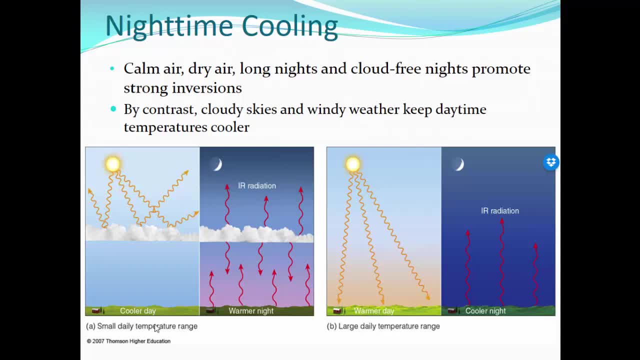 nights. That allows the earth to cool very quickly. So look at the far right. Infrared radiation is escaping to space very easily on a clear, calm, dry night. Look on the left: The warmer night cloud cover both absorbs and re-radiates away infrared radiation, and that. 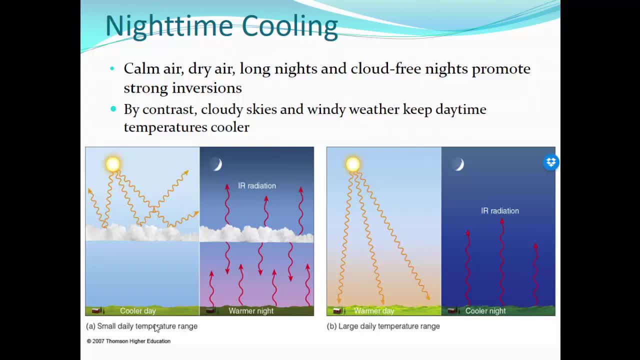 night will be warmer. It's the opposite with the daytime. In the daytime, calm air, clear skies, even dry conditions, We'll allow all of the sun's incoming solar radiation to strike the earth and make for a warmer day And, as we talked about in chapter two, with cloud cover, whether it's scattering. 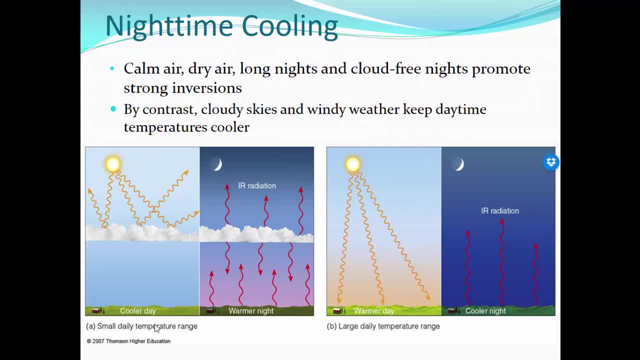 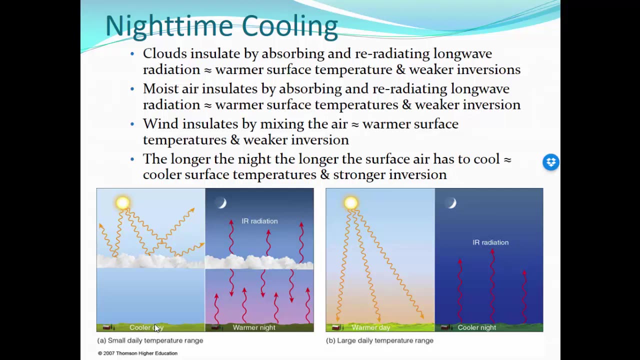 or reflection or even absorption. those three occur with the incoming solar radiation and not as much of that insulation reaches the ground and therefore you have a cooler day. Same general illustrations: Nighttime cooling Clouds insulate by absorbing and releasing re-radiating long-wave radiation. Therefore warmer surface temperatures, weaker inversions. 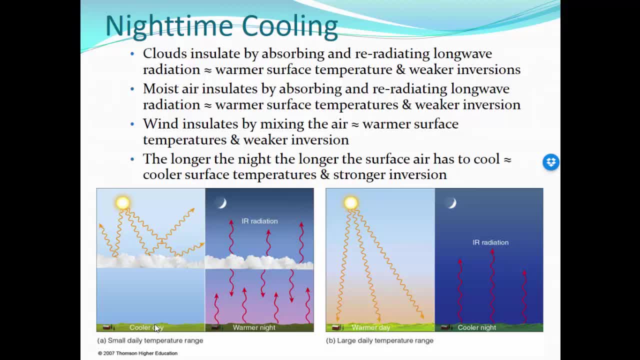 The temperature difference between the very cool surface and the slightly warmer six feet above ground level is not as high. Moist air insulates by absorbing and re-radiating long-wave radiation, So with high humidity you're going to have warmer surface temperatures. 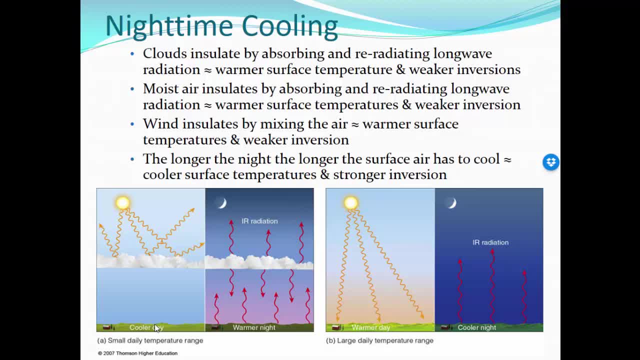 at night. Wind insulates by mixing the air, And so when you have windy conditions, you'll have warmer surface temperatures at night. Of course, the longer the night is, the longer the surface has to cool, So a longer night will provide for cooler surface temperatures. 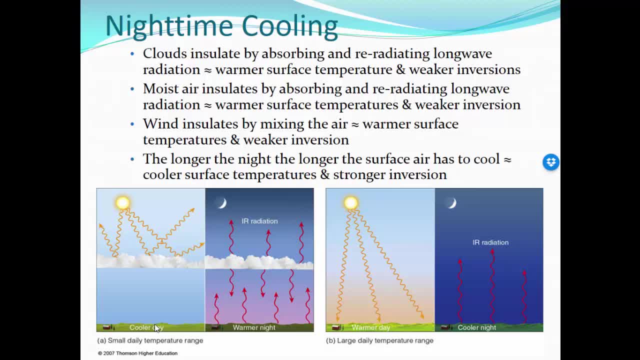 So each factor has a different impact: Clouds during the day, keeping it cooler. Clouds at night, keeping it warmer. Clear skies during the day- making it warmer. Clear skies at night, making it cooler. Wind during the day: makes it feel a little bit cooler. A windy. 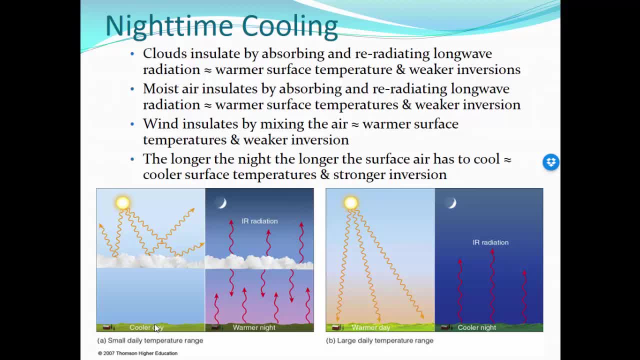 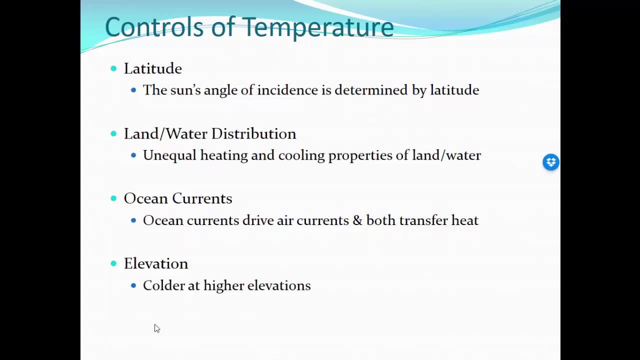 day is going to feel a little cooler, Wind at night mixes the atmosphere up, cooling does not happen as efficiently And windy nights tend to be a little bit warmer. What are the controls of temperature on a global scale, even a regional scale? Well, 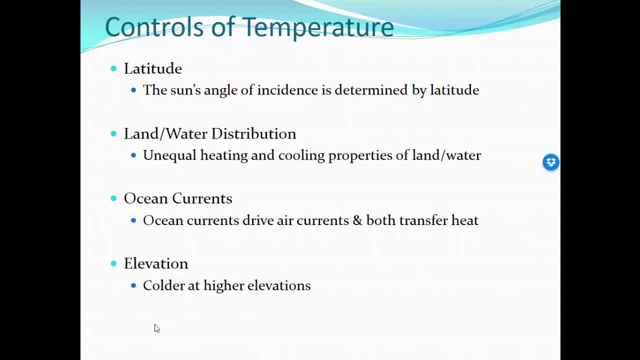 we have four of them: Latitude, land water distribution, ocean currents and elevation. Latitude refers to the sun's angle of incidence as determined by latitude. The higher the angle of incidence, the more warming capacity of the sun's rays, The highest angles of incidence being at lower latitudes such as the equator. 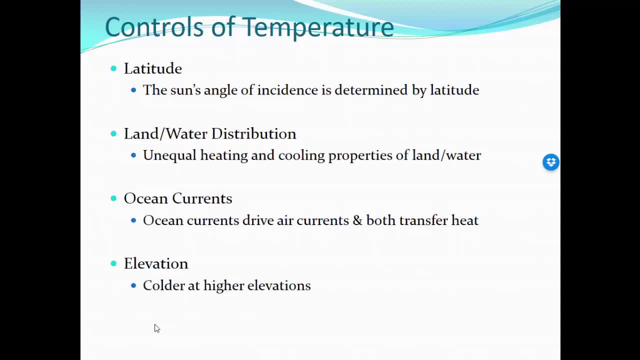 Land water distribution is another control of temperature. The unequal heating and cooling properties of land and water have a big impact on the climate of a region. Land heats up and cools off much more quickly. Both heats up and cools off much more quickly. 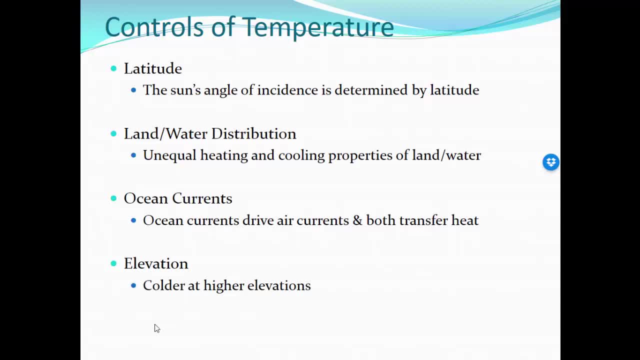 than water, Because water heats up and cools off much more slowly. areas near large areas, Large bodies of water have a moderate climate. They don't get as cold, but they also don't get as warm. Land water distribution and the unequal heating and cooling properties of land and water being 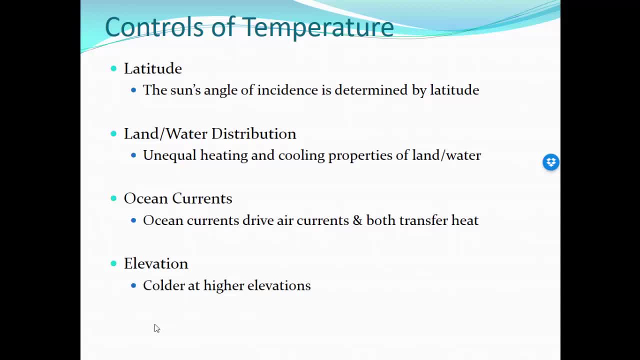 a major control of temperatures. Ocean currents also a major control of temperatures. Ocean currents drive air currents, warm air currents, north, but also transfer heat, with warm ocean water being moved to the north. Ocean currents can have a big impact on entire regions of the world. 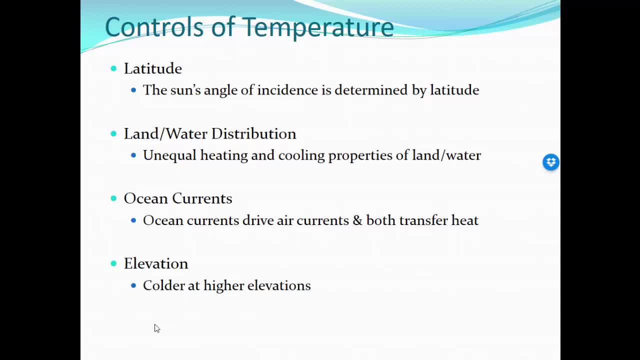 You can think about Western Europe, including England and Scotland and Ireland. Those are at very high latitudes, the same latitudes of northern parts of Canada, but they are much, much warmer year round because the Gulf Stream current, which we'll show, 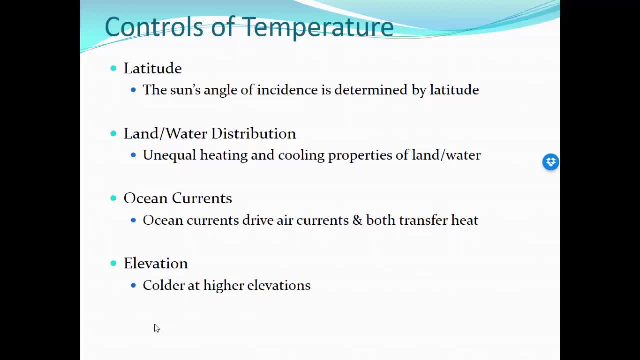 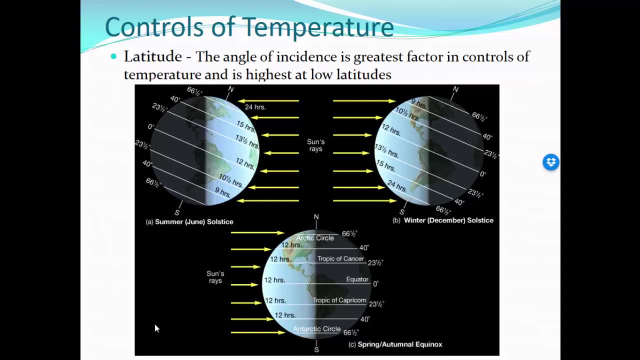 you in a few minutes, brings warm water to those areas. And elevation acts very similar to latitude. We're at higher elevations, you're colder than at lower elevations. So the first control of temperature. this is a very good description of latitude. 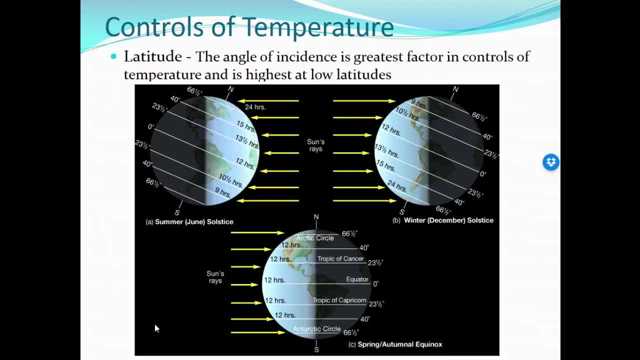 So A is the summertime, the northern hemisphere is tilted toward the sun, B is the wintertime, the northern hemisphere is tilted away from the sun, And C is spring and autumn. So A represents the summer solstice, B represents the winter solstice, C represents either the 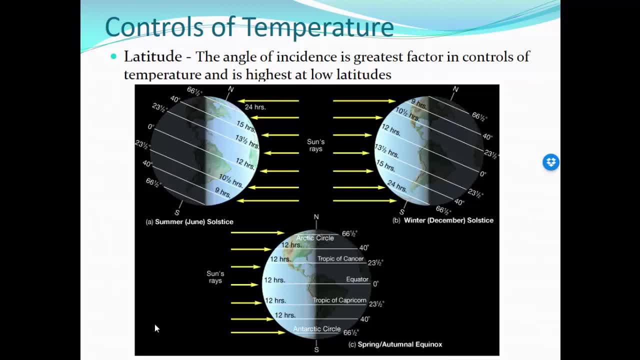 spring or the autumnal equinox. And again, equinox refers to the fact that on those days there are equal parts of day and night, 12 hours of day and night. And you can see, in our summertime our days are long, 13 and a half to 15 hours long in. 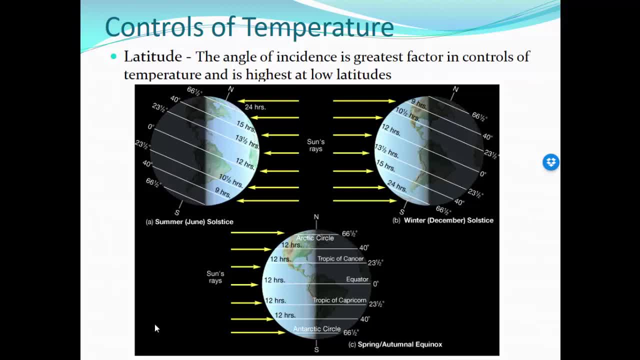 North America And in our wintertime. our days are much shorter, somewhere between 9 to 10 hours in North America in our wintertime, But at the equinoxes both of our day and night are 12 hours. 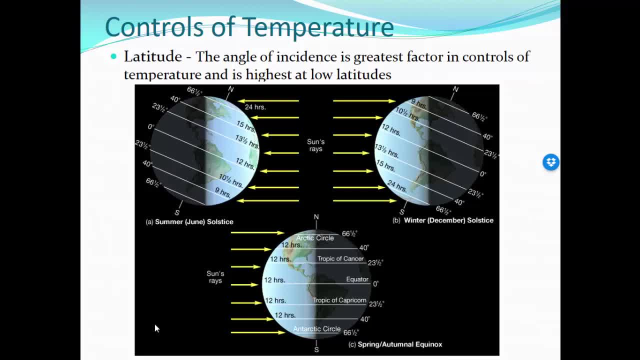 More important than the length of the daytime. the length of the daytime, of course, is a control of temperature, but the angle of incidence, the angle at which the sun's rays strike the Earth. Look at C, at the equator, those sun rays strike at a 90-degree angle. 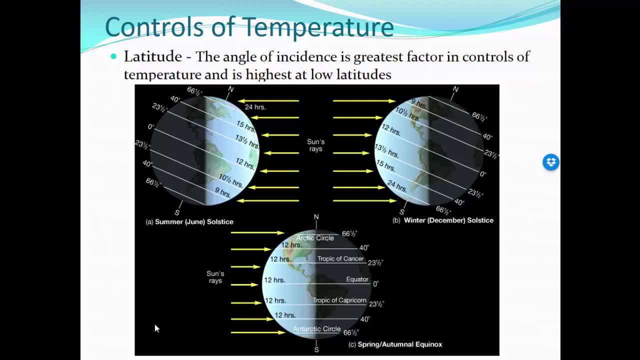 The higher the angle, the more warming capacity of those sun's rays, And even at the Arctic Circle and the North Pole the angle is not terribly small, And so that's why, in the summertime, the Arctic Ocean actually will melt. 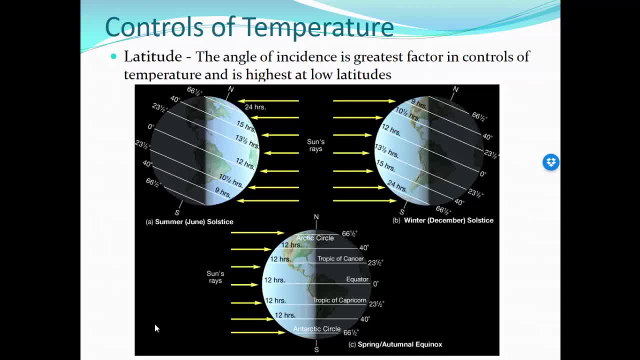 And it's not warm at the North Pole, but it's also not sub-freezing the entire time, Conversely, in the wintertime. look at B and look at the Arctic Circle. The Arctic Circle in the winter, at the winter solstice, is completely dark. 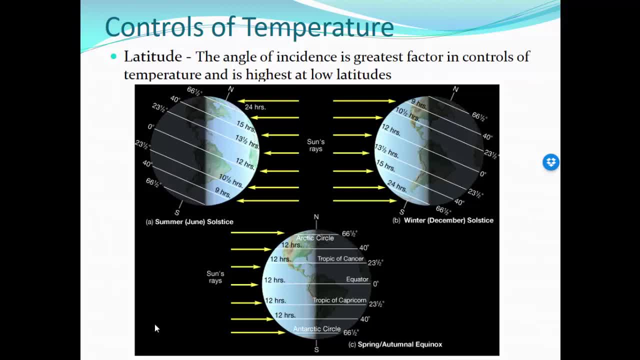 That's where you get the six months of winter. It's tilted away from the sun. So not only are the sun's rays almost at a tangent to the globe there, in some cases, north of the Arctic Circle, they don't strike the globe at all. 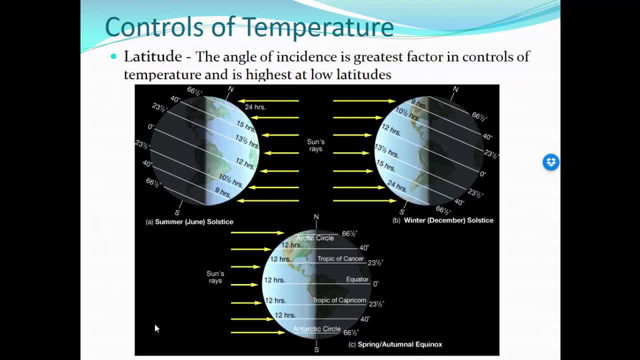 Six months of nighttime and so obviously very cold, Where in our summer the sun's rays do strike the North Pole, but they don't strike the South Pole. So the angle of incidence is the greatest factor in controls of temperature and is highest. 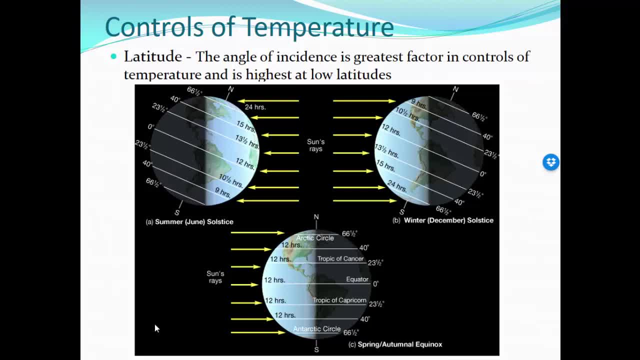 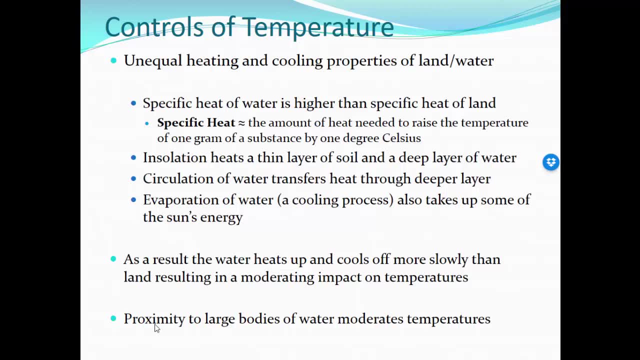 at low latitudes. That angle of incidence is highest at low latitudes. Unequal heating and cooling properties of land and water. Specific heat of water is higher than specific heat of land. The specific heat is the amount of energy needed to raise the temperature of one gram. 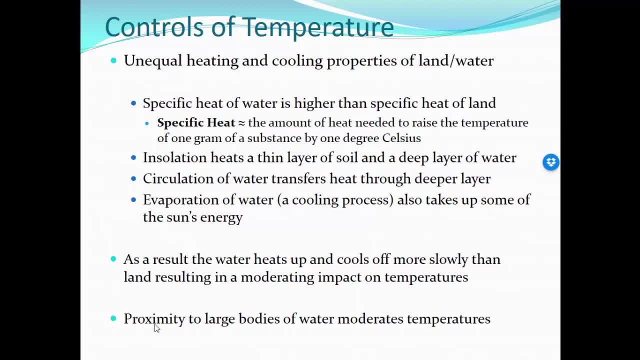 of a substance by one degree Celsius. We know that it takes one calorie of heat to raise one gram of water by one degree Celsius. Most other substances require less heat than that, So water requires the most heat to heat up, But it also requires the removal of more heat to cool off. 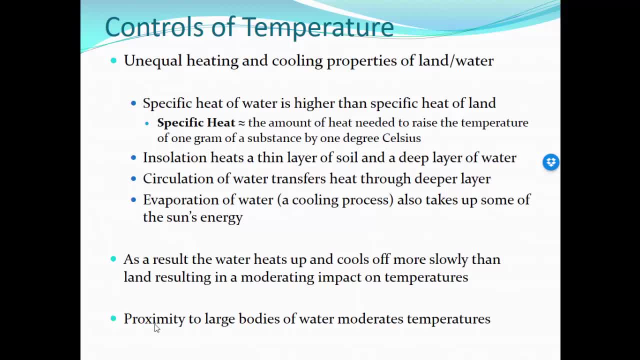 So that's the first reason why water heats up and cools off more slowly than land: The specific heat of water. The second reason that water heats up and cools off more slowly than land is that insulation, incoming solar radiation or incoming shortwave radiation, only heats a thin layer of soil. 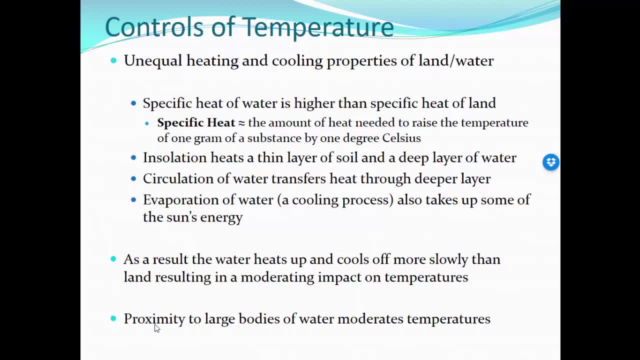 Meaning it only has to heat that very, very far. That's the first thin layer of soil, Whereas the rays of the sun penetrate and have to heat a much deeper layer of water. So the sun is much more efficient at heating the earth than it is at heating water. 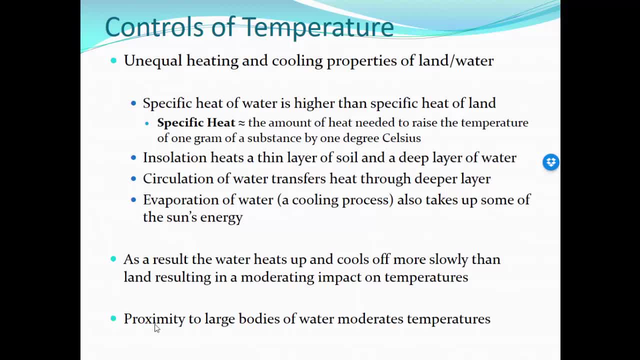 And therefore water. again. the world's oceans and large lakes heat up and also cool off more slowly than land. Also, with land soil there's no circulation, Meaning the cold rocks six feet under stay cold and six feet under, Whereas with the ocean and even lakes, 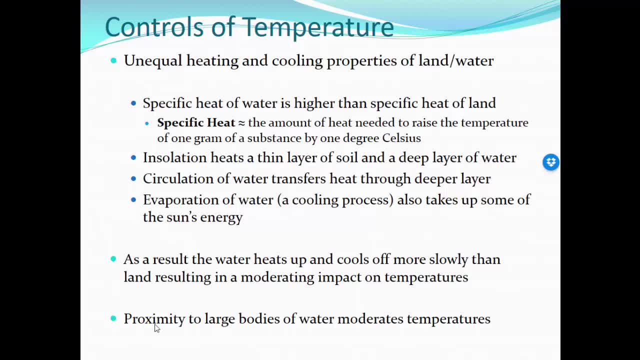 If it's colder Six feet below the surface, Circulation of water tends to move that water around, And so the warmer water at the surface gets pulled to deeper depths. The cooler water at the deeper depths gets pulled to the surface, and it takes much more. 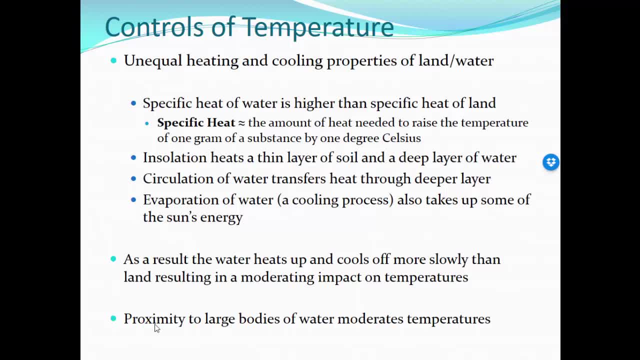 heat to warm up an ocean or a lake or a gulf, The last going back to latent heat, and remember that evaporation is a cooling process. The opposite, condensation, is a warming process, but in this case evaporation is a cooling process. 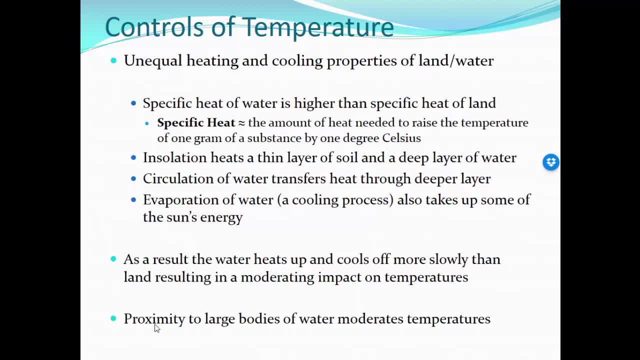 And that also takes up some of the sun's energy. So energy. So main reason: these four reasons, the main reason why the oceans and the lakes and the gulfs heat up and cool off more slowly than the earth. So, as a result, the water heats up, cools off more slowly than land, resulting in a 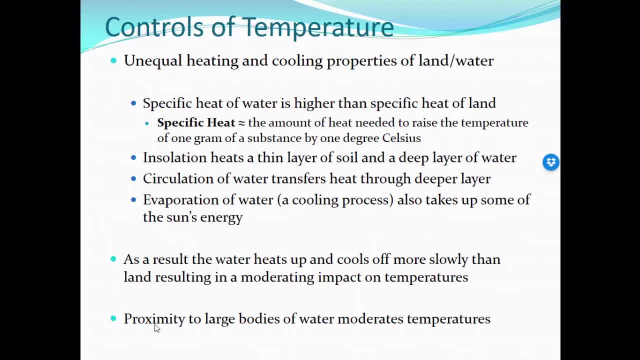 moderating impact on temperatures, proximity to large bodies of water, moderate temperatures: It doesn't get as cold in the wintertime, but it also doesn't get as warm in the summer. Think about Seattle. In this situation, we can see that St Louis 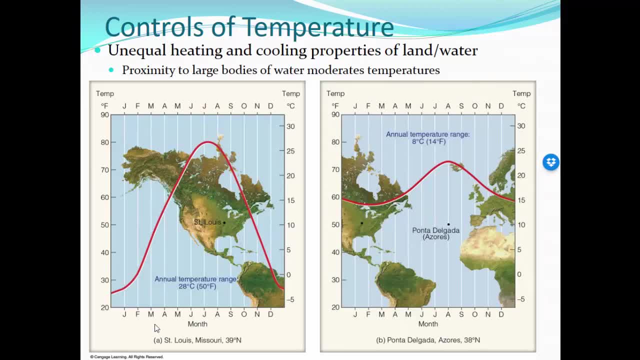 And And Ponto Delgada are essentially at the same latitude by the same place north of the equator, But we can also see that in St Louis we have a high variation in seasonality, meaning quite chilly in the wintertime but also again quite hot in the summertime. 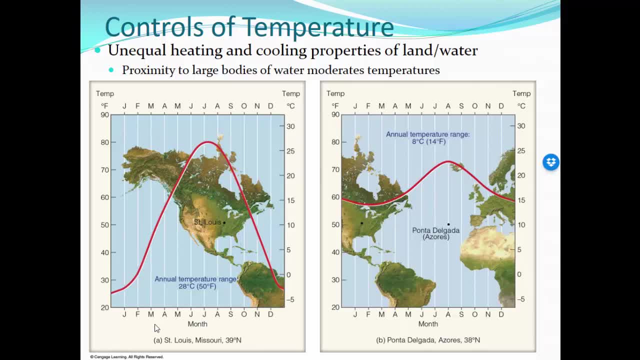 It's in the middle of a continental landmass, a long way from any large body of water, whereas a small island in the middle of the ocean. the temperatures there throughout the year moderated, And that's significantly by its proximity to that large body of water. 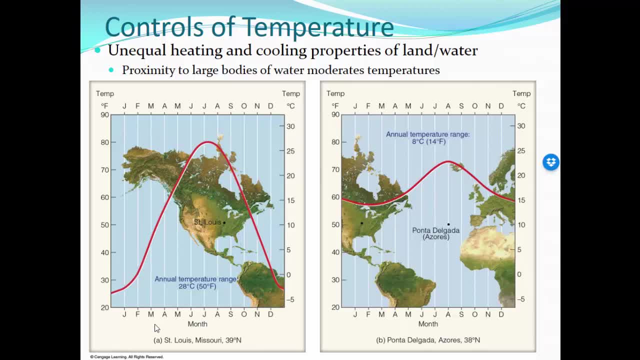 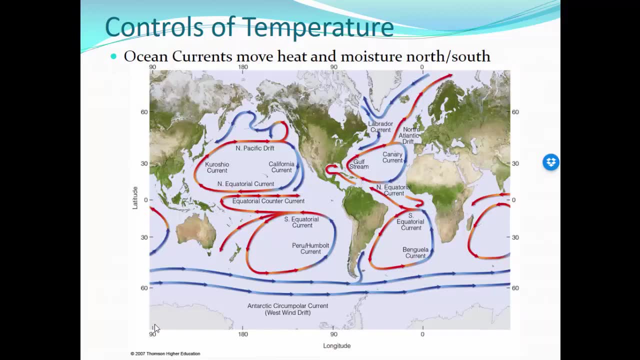 Not quite as hot in the summertime and certainly not as cold in the wintertime. Ocean currents as a control of temperatures. So these are the great ocean currents of the world. There are five, what we refer to as gyres, G-Y-R-E-S. 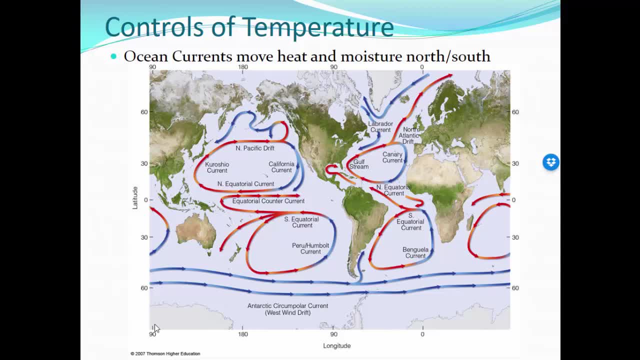 One in the North Pacific, one in the South Pacific, one in the North Atlantic, one in the South Atlantic And one huge one, One between Antarctica and South America, Australia and Africa and Indonesia and South Asia, called the Antarctic Circumpolar Current. 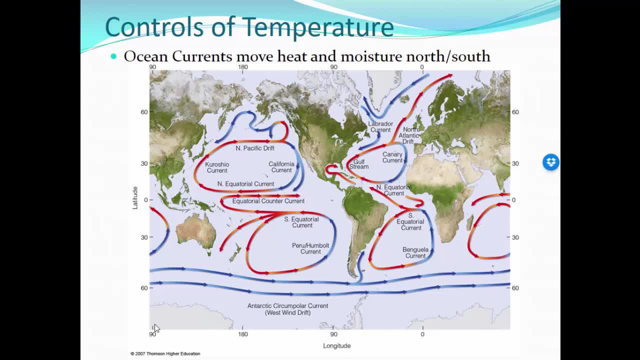 We're not going to concern ourselves too much with that one, Just the first five. And you can see that all five of those move clockwise across the ocean basins And you can also see, looking at this, just how much larger the Pacific Ocean is than. 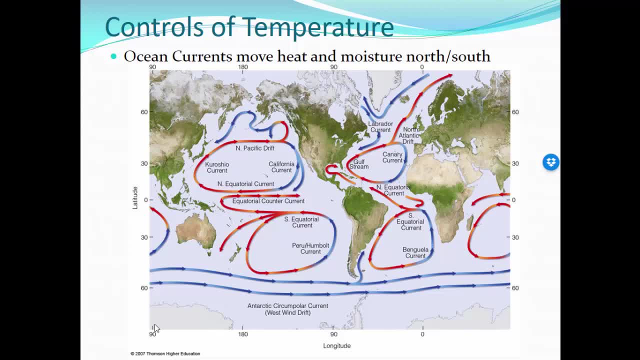 the Atlantic and the significantly larger body of water, The clockwise flow of water around the North Pacific Ocean. The Atlantic is the largest body of water in the entire Pacific Ocean. The Atlantic is the largest body of water in the entire Pacific Ocean. The Atlantic is the largest body of water in the entire Pacific Ocean. 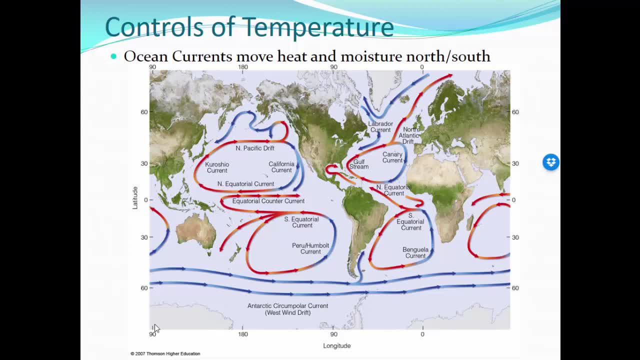 The Atlantic basin means water moving from Indonesia. at the equator It's very, very warm, keeping Japan fairly warm. But as that water moves across the North Pacific it cools, And as it moves along the west coast of North America it keeps the west coast of North. 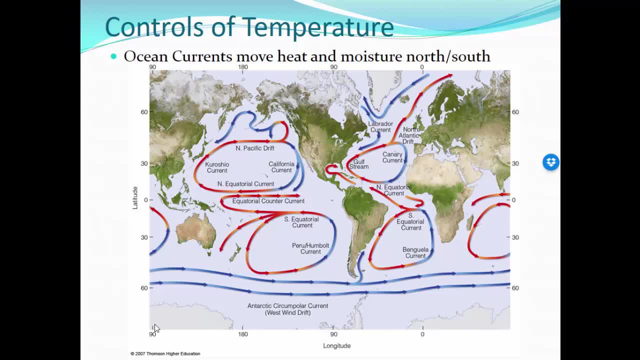 America fairly cool. Think about going in the Pacific Ocean if you've ever had the chance. It is so much colder, even in the summertime, than the Atlantic Ocean. As a matter of fact, Mark Twain said the longest winter he ever seen. 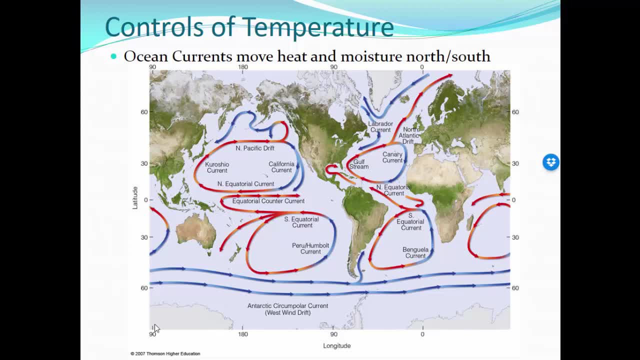 he ever spent was one summer in San Francisco, because that cold California current keeps San Francisco and Central California very, very chilly, even in the summertime. The opposite occurs in the Atlantic Ocean, because we are on the west side of the ocean basin, the east side of the continent, the west side of the basin. 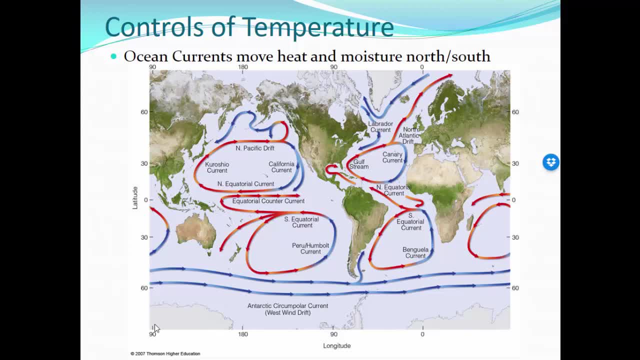 And again that Gulf Stream, nice and nice and toasty warm, And as it moves by Florida and the southern states it keeps our area very warm, very humid and really dramatically modifies our climate. But look at that warm water traveling across the North Atlantic. 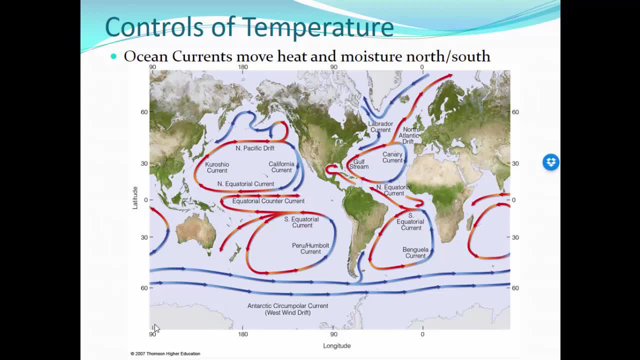 straight toward the Iberian Peninsula, the Bay of Iskay and the British Isles again, And that's why Western Europe, which is at the same latitude as northern parts of Canada, is so much warmer than North Canada because of that Gulf Stream. 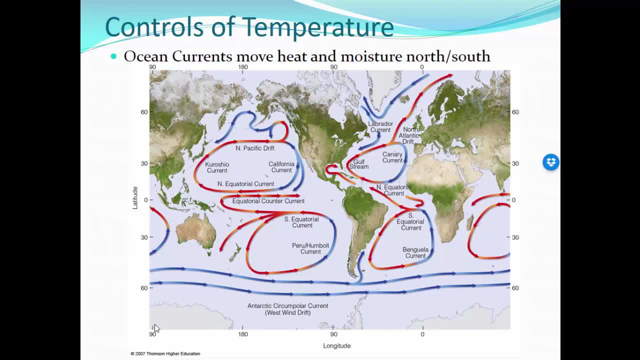 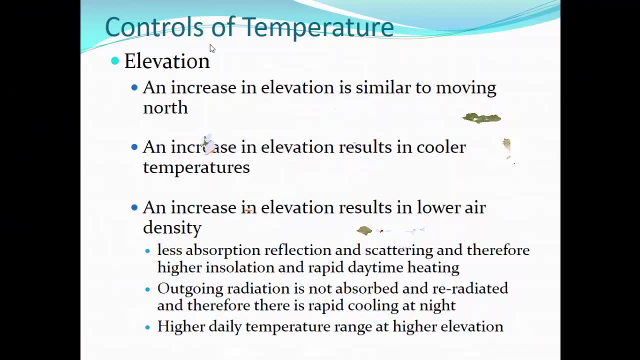 And the other effects also occur in the Indian Ocean, the South Atlantic and South Pacific as well. The last control of temperature is elevation. An increase in elevation is similar to moving north, So an increase in elevation is similar to an increase in latitude. 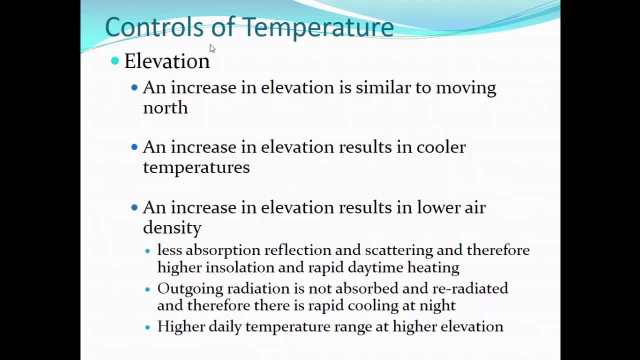 An increase in elevation results in cooler temperatures. An increase in elevation also results in lower air density. Remember, it's thinner up there. The air is thinner up there. As you go up in an airplane, the air is thinner. You may actually have to. 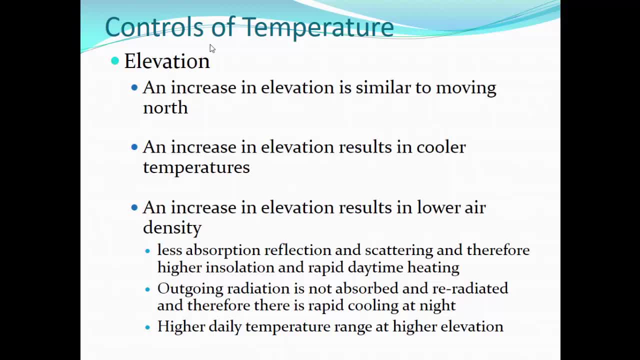 You use oxygen As you go up a mountainside, the air is thinner. If you decide you're going to train for an Ironman, do you train at sea level or do you go out to Colorado and train a mile high, where the air is thinner? 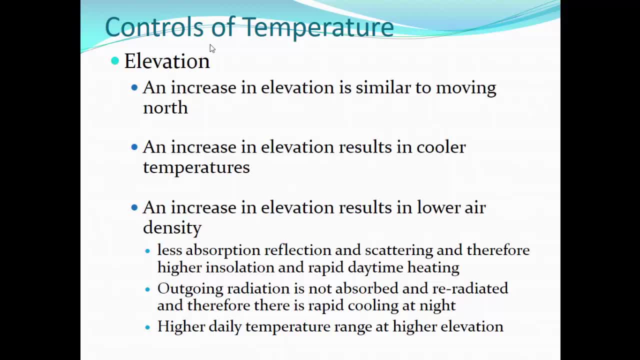 There's less oxygen. It makes you stronger. So because the air is thinner, there is lower air density. There are literally fewer molecules of air. at those higher elevations, A couple of things happen that also moderate the temperatures at higher elevations. 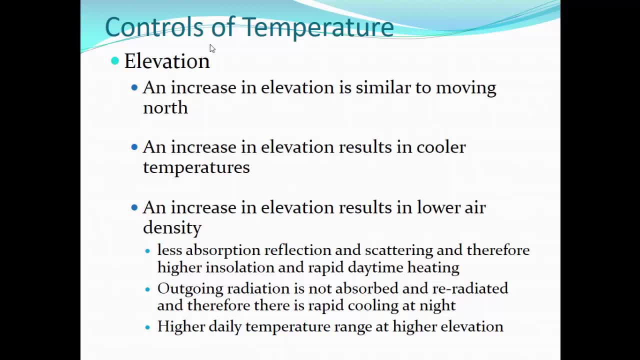 There is less absorption, reflection and scattering of incoming sources of solar radiation, So less of the sunlight is absorbed, reflected or scattered as it strikes the Earth during the day. That means that temperatures heat up very quickly at higher elevations. Now they may not get very warm. 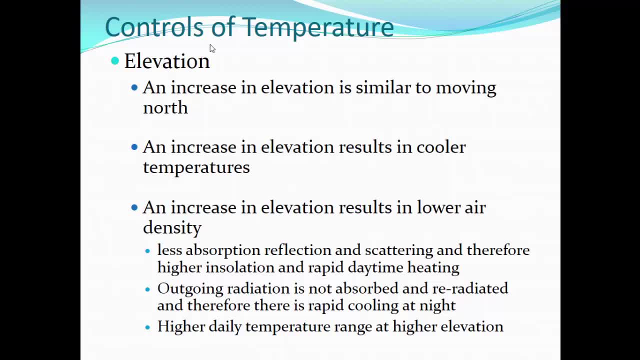 but it goes from the very cold minimum temperature to the maximum temperature of the day very, very quickly at higher elevations. Also, outgoing radiation- this is at night- is not absorbed and re-radiated and therefore there is rapid cooling at night. 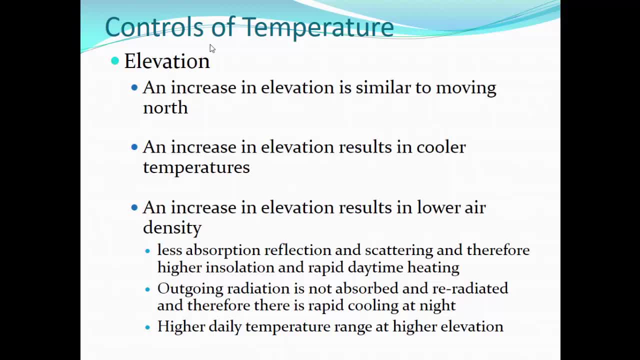 So both rapid heating during the daytime and rapid cooling at night. And that is why our high elevation deserts of western parts of Texas and into New Mexico and Arizona, those high elevation deserts are very, very cold at night and very, very warm during the daytime. 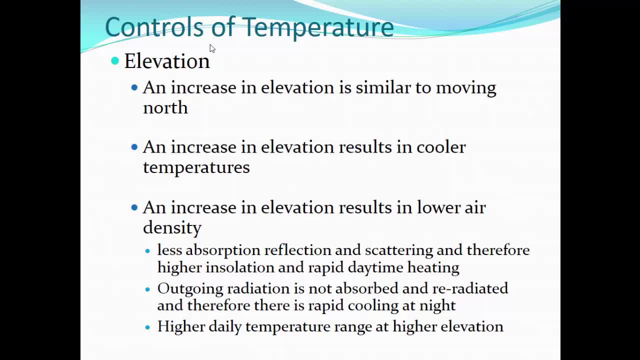 because at night the temperature falls very quickly without all that air, those air molecules to absorb and re-radiate, And at night it gets very chilly. And then in the daytime, without those air molecules to reflect, scatter and absorb. 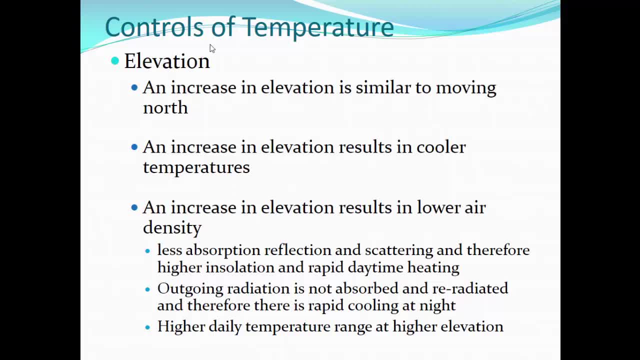 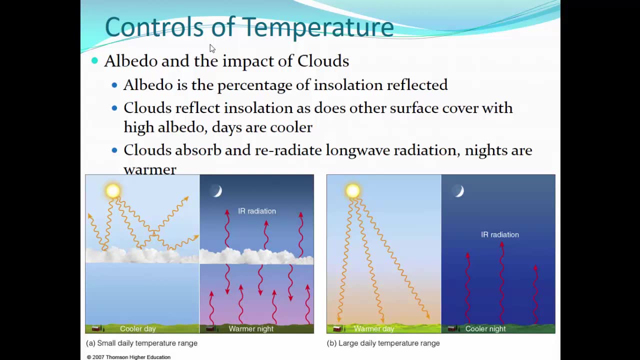 temperatures heat up very quickly, So there is a higher daily temperature range when you are at higher elevations. Now we've seen these pictures before: Controls of temperature, Albedo and the impact of clouds. Remember albedo is how much light is reflected. 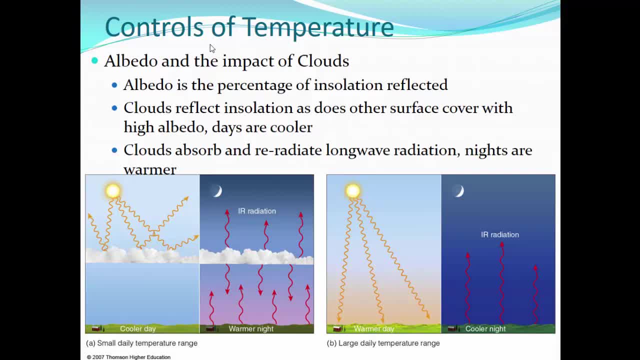 directly back from a surface And thick clouds had high albedo, They reflected a lot of light back. Albedo is the percentage of insulation reflected. Clouds reflect insulation, as do other surface cover. with high albedo, Days are cooler, So what does that mean? 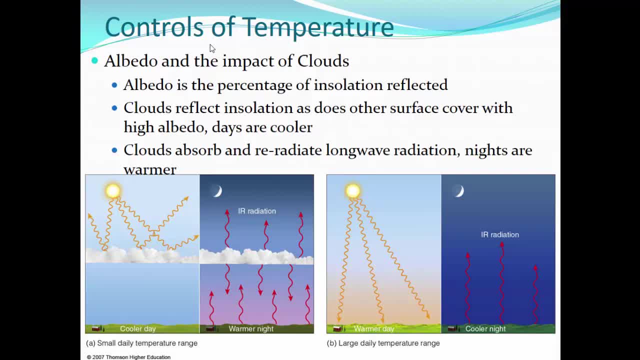 If there's high albedo, thick clouds or surface cover that has high albedo, your days will be colder Again. last lecture I mentioned fresh snow has very, very high albedo, Reflects more than 90% of the sunlight back. 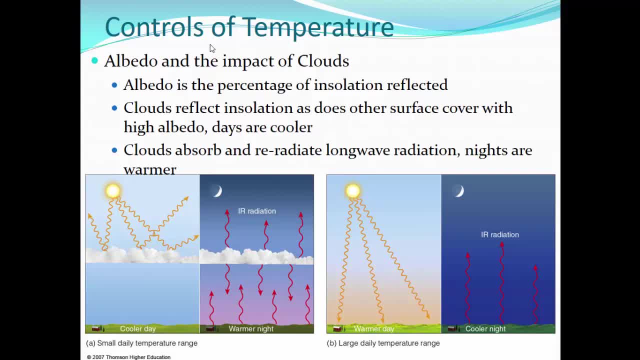 And so fresh snow will keep temperatures colder than literally old snow. If you take fresh, crisp white snow, it's going to reflect all that light very easily If you go down into an urban area where the snow has had a chance to partially melt. 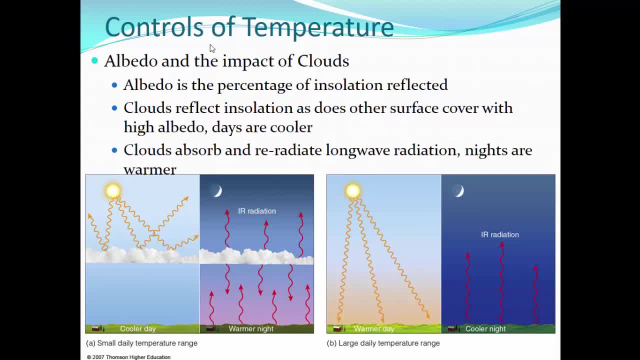 and it's gotten dirty and gray. it doesn't have very high albedo at all, So clouds reflect insulation, as does other surface cover. with high albedo and days are cooler, Clouds also absorb and re-radiate long wave radiation. 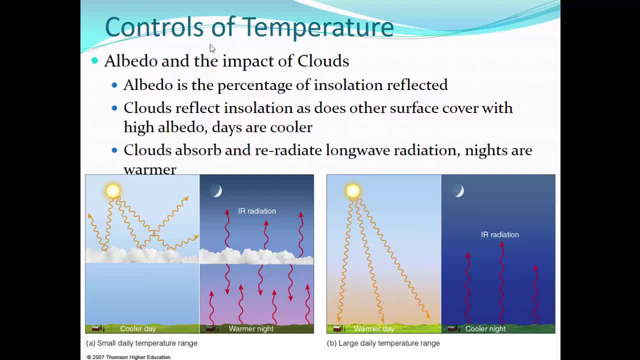 Remember, the Earth is radiating away its heat, its infrared radiation, its long wave radiation. The Earth is radiating that away 24 hours a day, daytime and nighttime, And at nighttime, if the skies are clear, it very easily radiates its energy away. 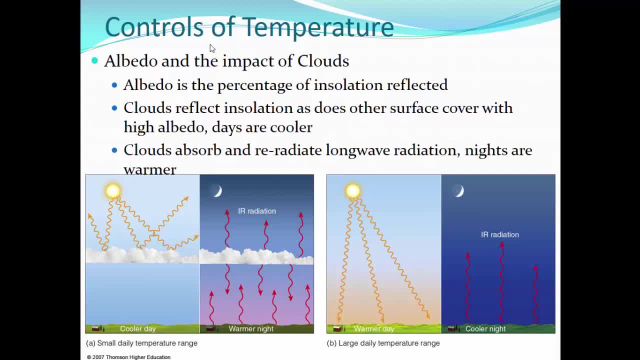 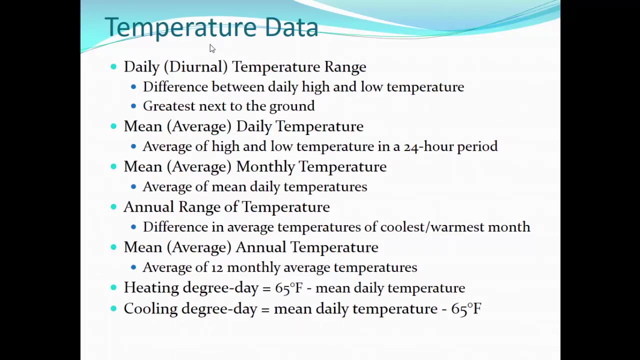 But if there are clouds at night, those clouds absorb and re-radiate long wave radiation and our nights are warmer- Temperature data- And this applies more to climatology and the nomenclature of climatology- what people are talking about when they say different things? 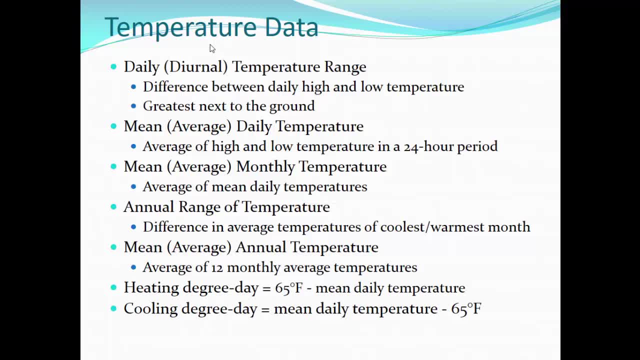 Let's go through this quickly. This is all in your book. The daily or diurnal temperature range is the difference between the daily high and low temperature, And it's again greatest next to the ground. Now you've probably heard the term nocturnal. 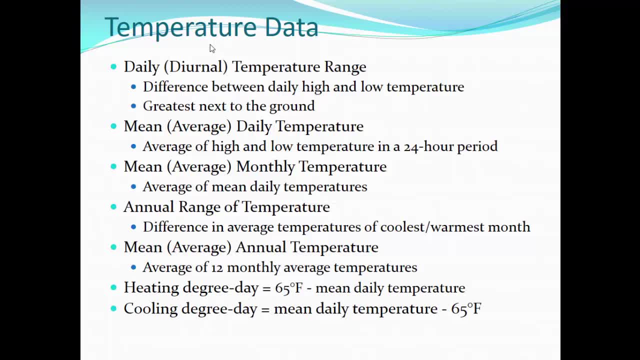 If you have a cat you may know your cats are nocturnal. They run around at night. Diurnal is the opposite of nocturnal. It means during the day. So diurnal is the term in weather. that means during the day. So the daily temperature range: 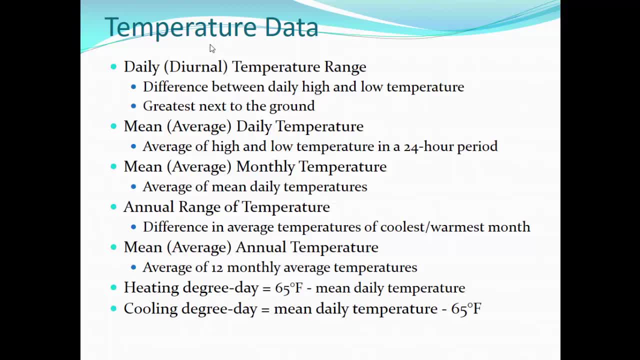 is the difference between the high and the low temperature. So if the daily temperature range in Florida was 30 degrees, that could mean the morning low was 60 and the afternoon high was 90. The mean daily temperature is the average high and low temperature. 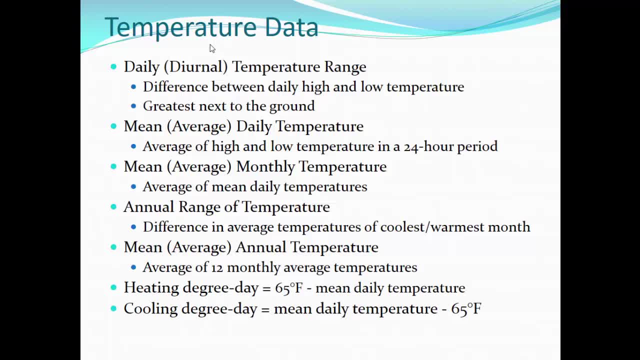 in a 24-hour period. So with that other example of 60 and 90, the mean or the average daily temperature for the day would be 75 degrees, the average of 60 and 90. The mean monthly temperature is the average of all those mean daily temperatures. 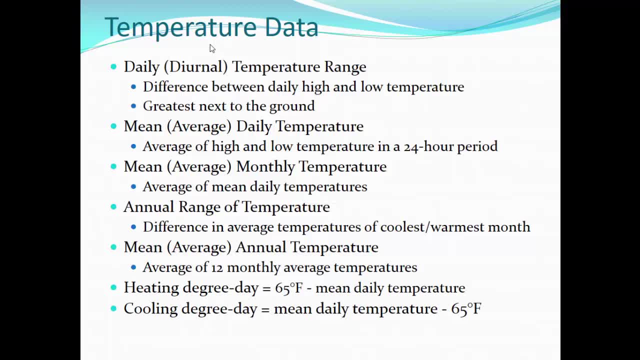 So let's just say, because it was a crazy month, every single day in the month had a mean temperature of 75, then the mean monthly temperature would also be 75.. The mean monthly temperature is an average of mean daily temperatures. The annual temperature range. 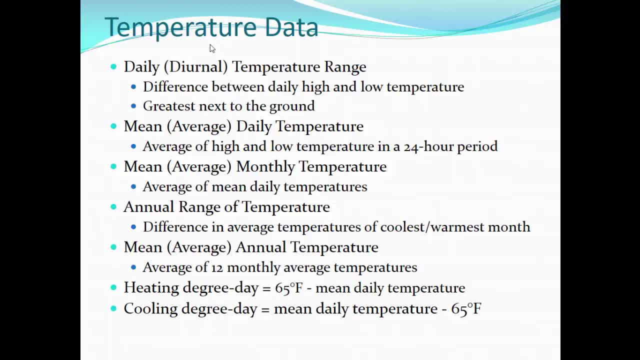 or the annual range of temperature, is the difference in average temperatures of the coldest and warmest month. So typically our coldest month will be January or February. Our warmest month will be August and September. The difference between the coldest and the warmest 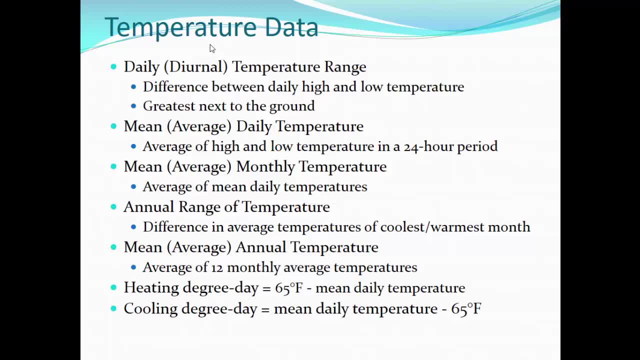 will be the annual range of temperatures for our area, And mean average annual temperature is the average of those 12 monthly average temperatures. Now, when it comes to energy and the purchase of oil and natural gas and coal for heating and for use in electricity for cooling, 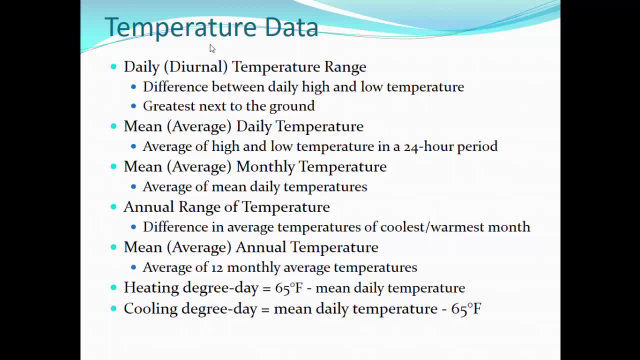 people that work in those markets refer to two terms: heating degree day and cooling degree day, And if the average temperature is more than 65 degrees, then let's say it is. the average temperature for a day is going to be 66 degrees. 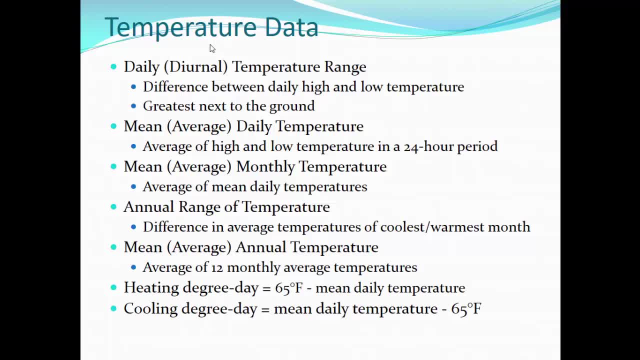 That is one cooling degree day. If the average temperature was 70 degrees, that would be five cooling degree days. So when people working in energy markets are looking at a seasonal forecast, they'll come up with a number. Maybe it's 250 heating degree days. 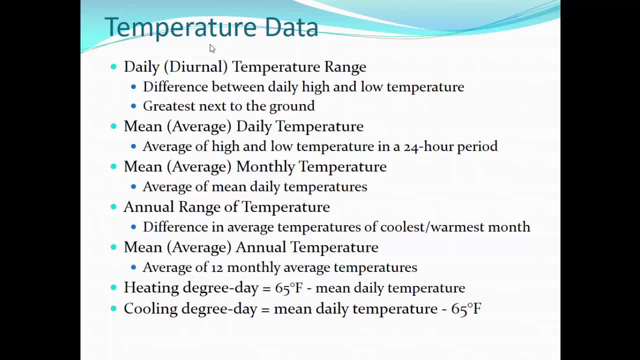 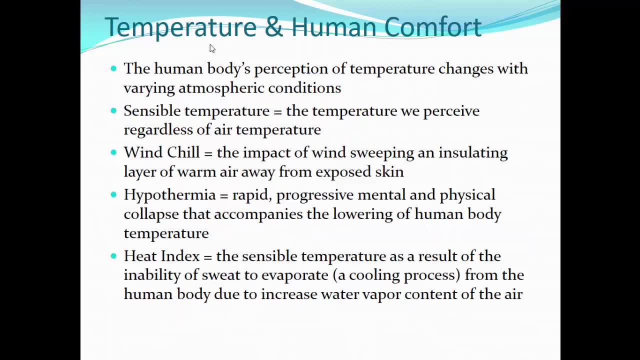 and that tells us how much natural gas or how much coal or how much oil they need to have for that upcoming season. So now we want to talk about temperature and human comfort. The human body's perception of temperature changes with varying atmospheric conditions, So the temperature may be 85,. 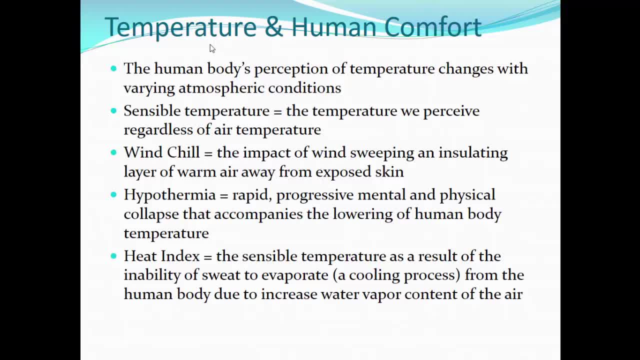 but it actually feels like it's 95 because of high humidity. Or the temperature may be 35, but it actually feels like 25 because of high wind speeds. The sensible temperature is the temperature we perceive, regardless of what the air temperature is. 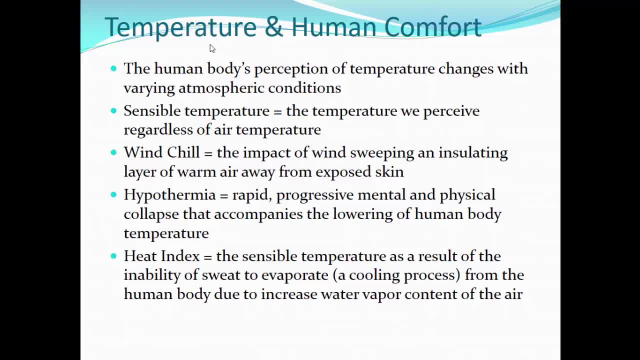 Two types: wind chill and heat index. Now, those are both human constructs, something that we've made up to define a phenomenon that we see in the atmosphere. In the case of wind chill, it is the colder temperatures we feel because of wind. 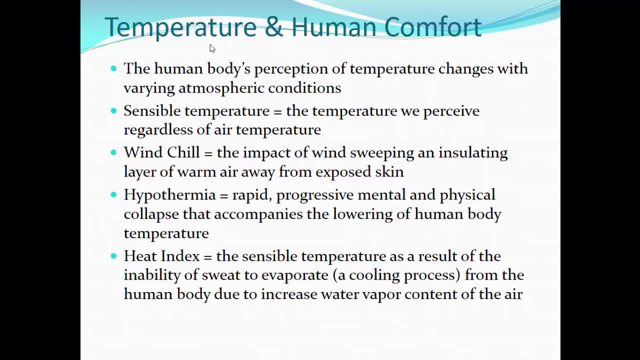 In the case of the heat index, it's the higher temperatures we feel because of high humidity. Wind chill is the impact of wind sweeping an insulating layer of warm air away from exposed skin. The body operates at 98 degrees plus It warms a layer of air around it. 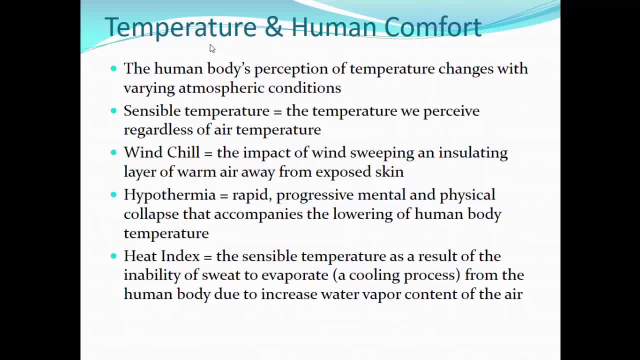 and that layer of air acts as an insulating layer. If it's windy and the wind can strip away that insulating layer, your body has to produce more heat in order to keep itself warm and we actually feel colder than the actual temperature. If this process continues, 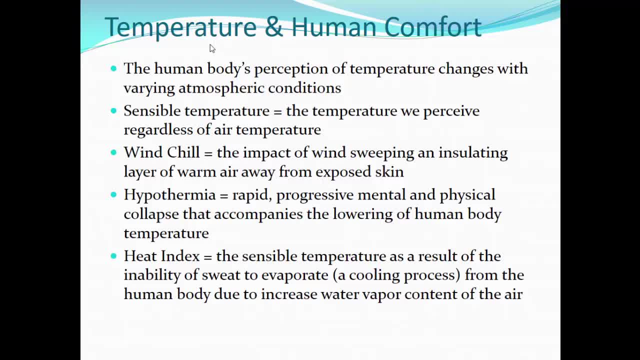 the whole body exposed to wind in a very cold environment, the rest of our body continues to be stripped away and our central temperature, our core temperature, human body's core temperature, falls far enough that hypothermia can set in, which is the rapid progressive. 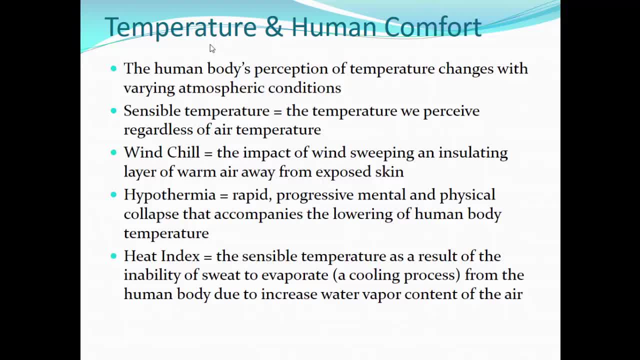 mental and physical collapse that accompanies the lowering of human body temperature. So wind chill is how much colder it feels because it's windy. but it has to be exposed skin, not something under a scarf or under a hat or under a jacket. It's all exposed skin. 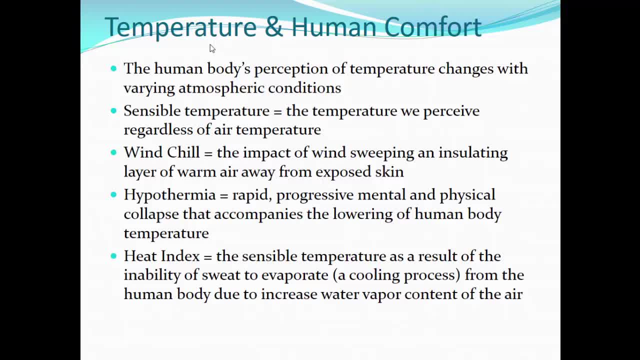 Your fingers, your lips, your nose, hopefully not your toes, but if they're exposed to the wind, they can have wind chill as well. Heat index is the opposite, and it occurs because of high water vapor content. Well, what's a better word for high water vapor content? 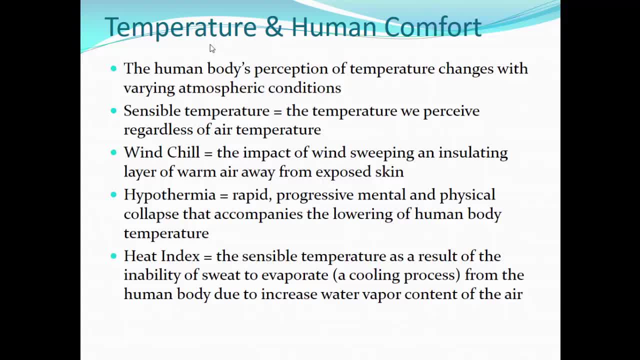 High humidity, The amount of humidity in the air. Water vapor is invisible. Look around the room. You don't see the water vapor in the room. There is humidity in this room. There is water vapor in the room. You just can't see it. 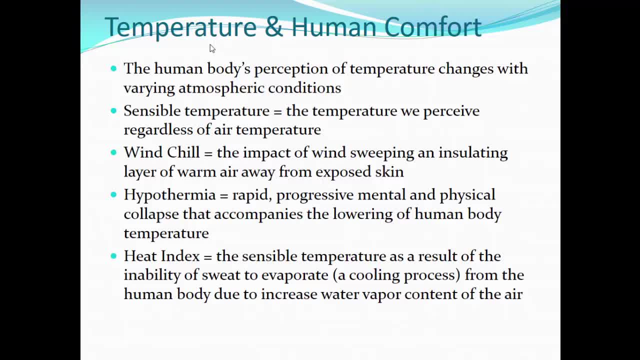 Look outside in the atmosphere, You don't see it there either. You do see clouds, but those clouds aren't water vapor, They are water droplets. So the higher the water vapor, the poorer the evaporative process is, meaning evaporation can't happen as easily. 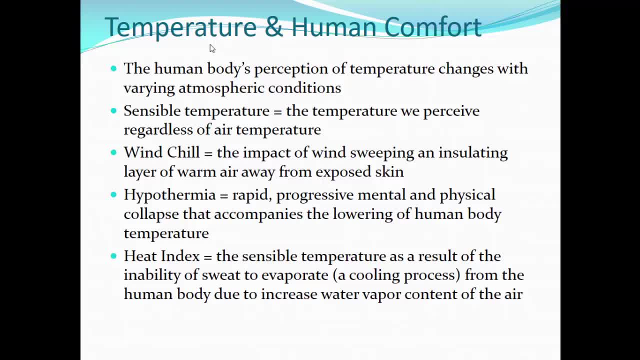 if there is high water vapor content. So why do we sweat? We don't sweat to get liquid on our bodies. That only makes us feel worse. when it's hot, Our clothes get damp and it's just well. it's icky. 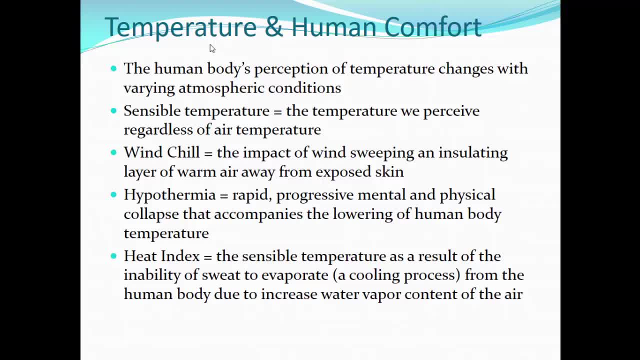 We sweat because the idea is for the sweat that goes out on your skin to evaporate And, as you know, evaporation is a cooling process. The heat index is the sensible temperature we feel as a result of the inability of sweat to evaporate. 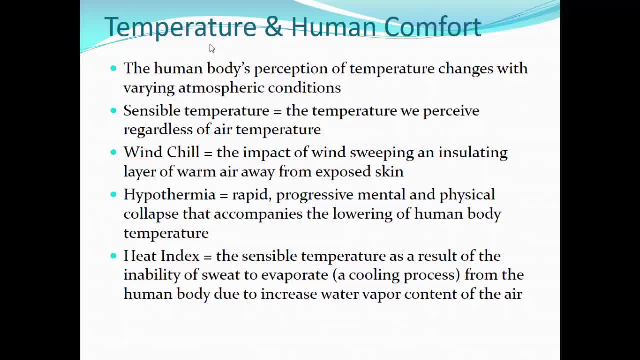 which is a cooling process from the human body due to increased water vapor content of the air. So 85 degrees with 95% relative humidity may feel like 100, where 85 degrees with 40% relative humidity may just feel like 85%. 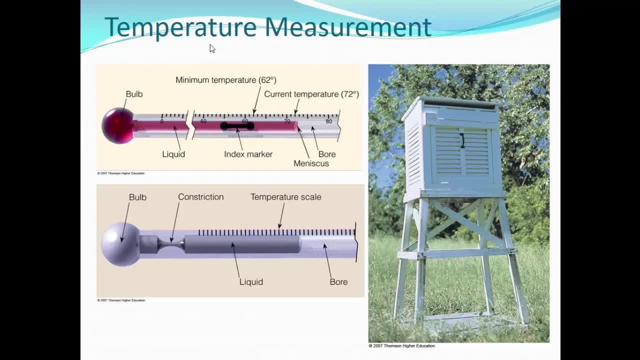 So again, here's your temperature measurement. There's lots of different types of thermometers and your book discusses these thermometers in detail. There's an actual picture of one of those temperature recording sites. You have your typical thermometer in the top, where your liquid- usually some type of a mercury. 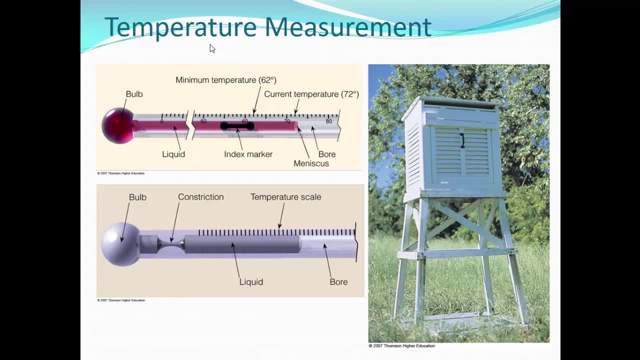 will climb up the thermometer when it warms up, That index marker will literally stay wherever it goes and that gives you an idea of the highest temperature of the day. Another way they get high temperatures is with this constriction thermometer where the mercury will go up the thermometer. 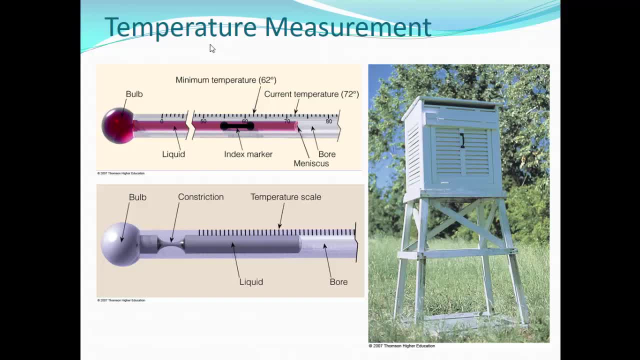 because it's constricted at the bottom, It won't come back down. That will also give you the highest temperature of the day. But there's lots of different types of temperature measuring devices, many of them now using electricity or also using lasers to determine the temperature of the air. 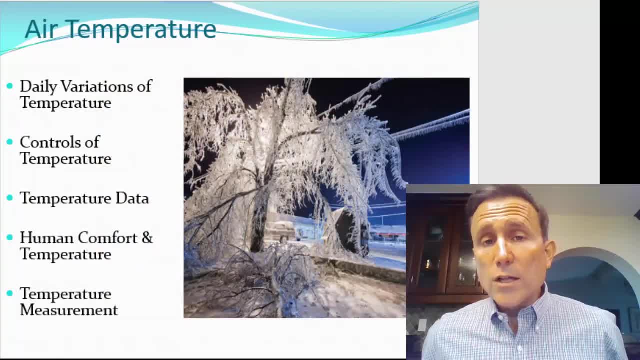 All right, that was Chapter 3 from Introduction to Meteorology. Next, Chapter 4, Humidity: Condensation in Clouds. What is humidity, What does it mean, How is it measured and what does it tell us? And then, once we know a little bit about humidity,